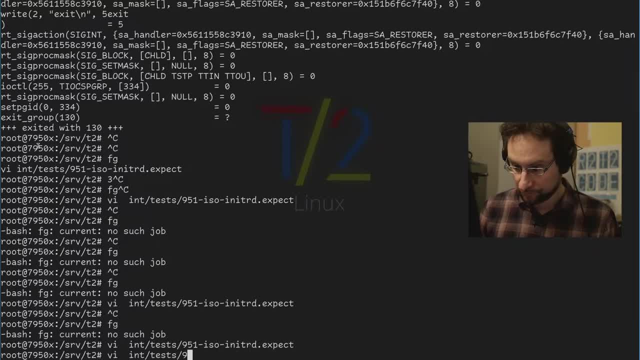 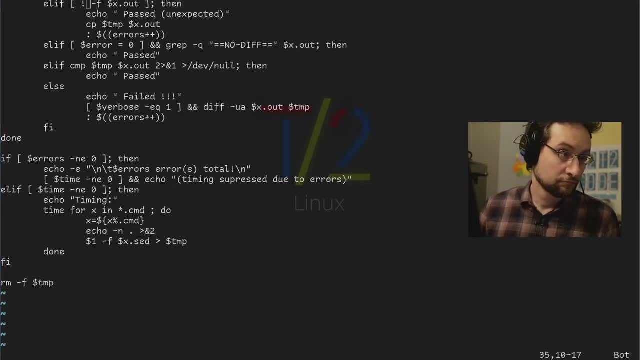 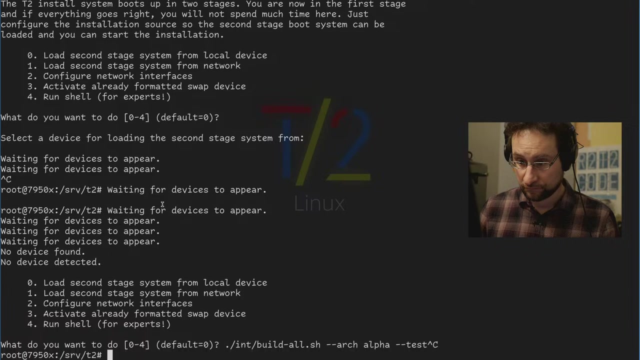 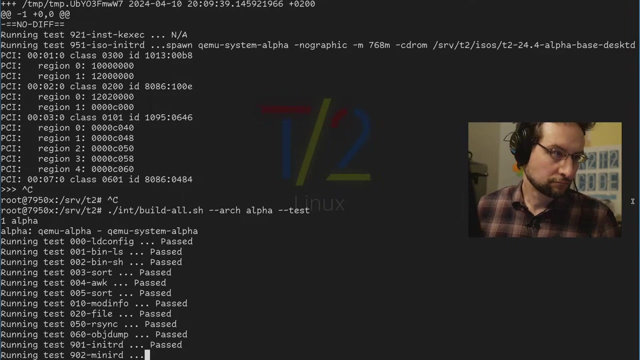 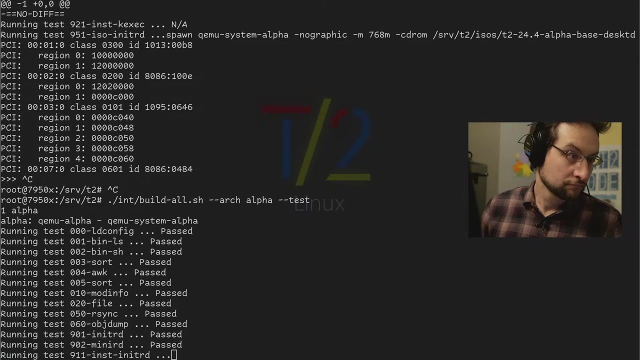 software and to permit persons software is furnished to do so, subject to the following conditions: the above copyright notice and this permission notice shall be included in all copies or substantial portions of the software. the software is provided. this is with our warranty of any kind express or implied coding, but not limited to the warranties of merchant ability. this 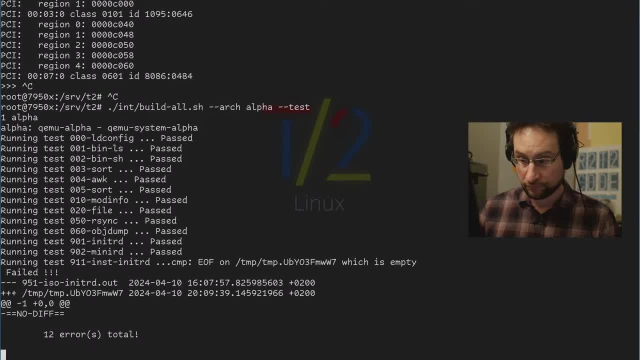 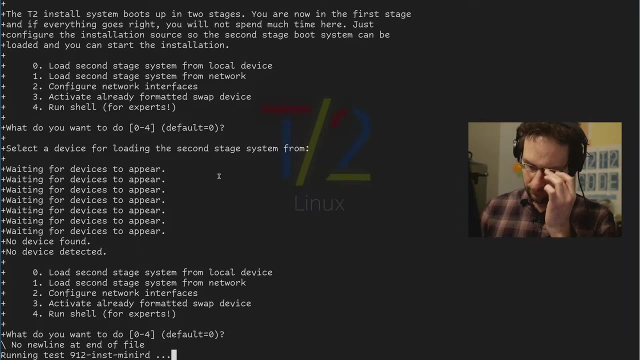 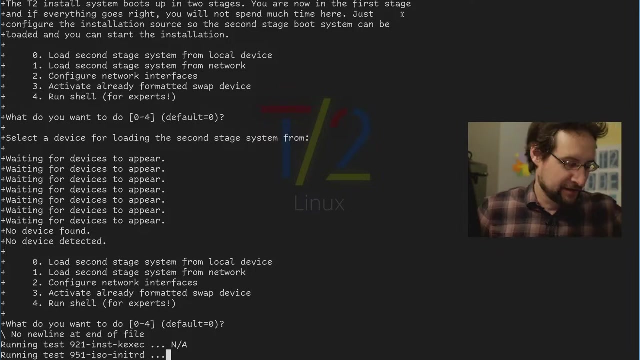 tip for a particular purpose and non-infraim it in no way and shall be all. welcome everyone, and thanks for artificial intelligence for this nice intro. currently i set it for years. so only substitute for testing is more testing and unfortunately we at least temporarily bricked some apple ibook. 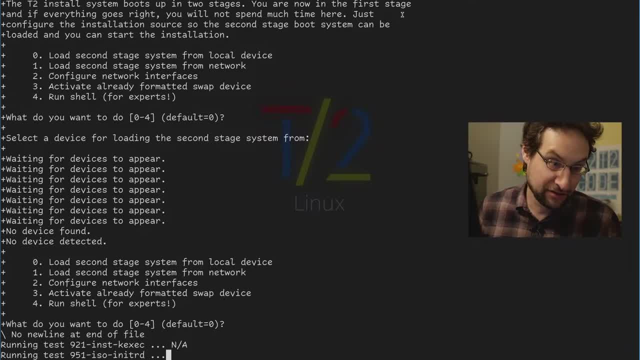 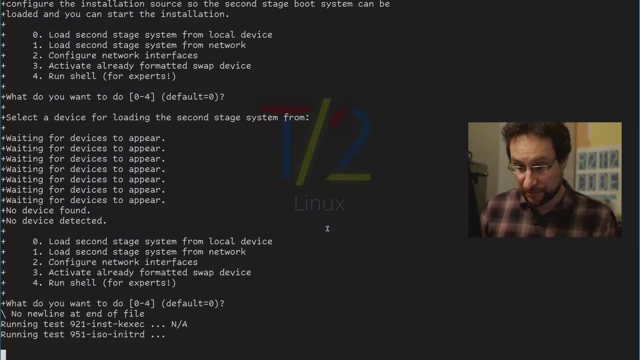 despite all our efforts and testing, unit testing, more unit testing. as a consequence, we stepped up more unit testing here. we previously started that testing the open source world, and now we tested more. so you can see, also slightly wonder why this doesn't test, but i don't know why it doesn't test, but i don't know. 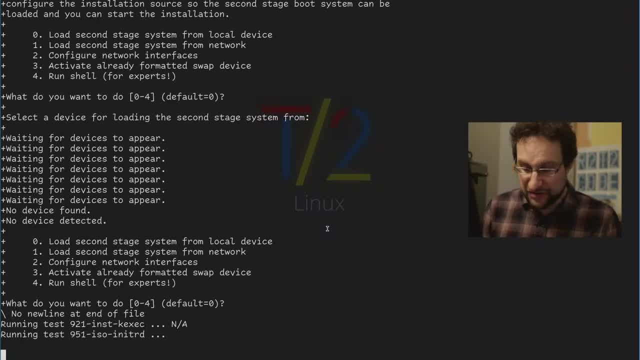 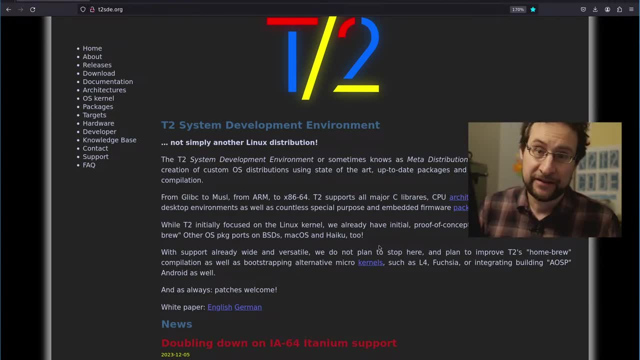 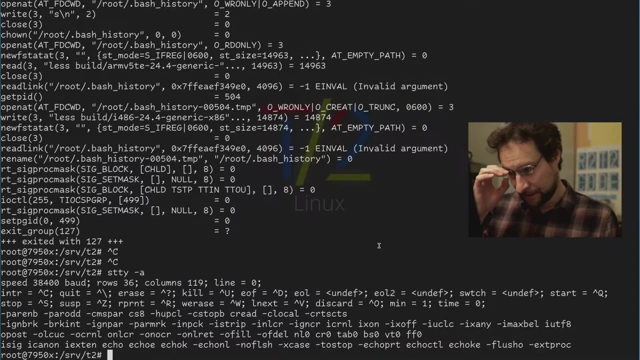 I guess whatever. Previously we started this, so we built this Linux distribution. right, If you're new to our channel, we for 25 years built one of those minimally working just pure Linux for architectures including PowerPC and stuff, P3 and all the other MIPS. 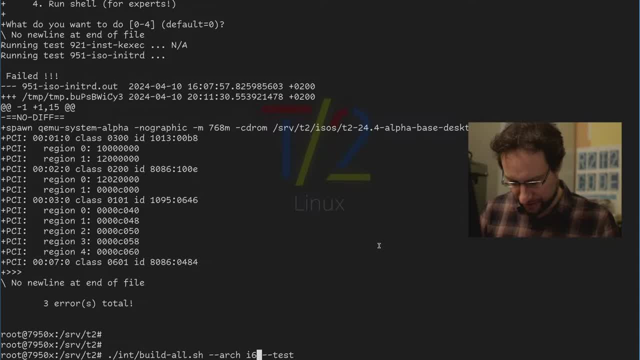 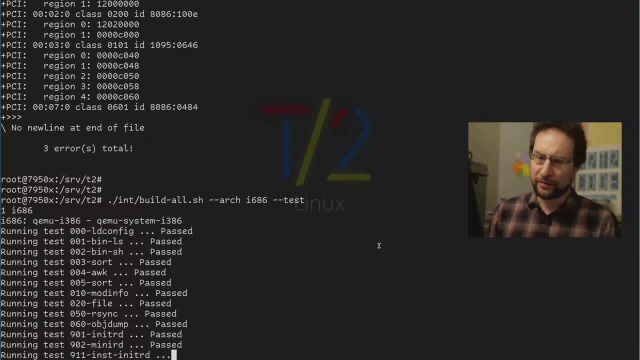 and so on, And of course, we wanna test this, and that is what today, for many hours, live on Twitch. we worked on this Previously. if you're new to this or if you're a working subscriber, you've seen my increasing test suite. 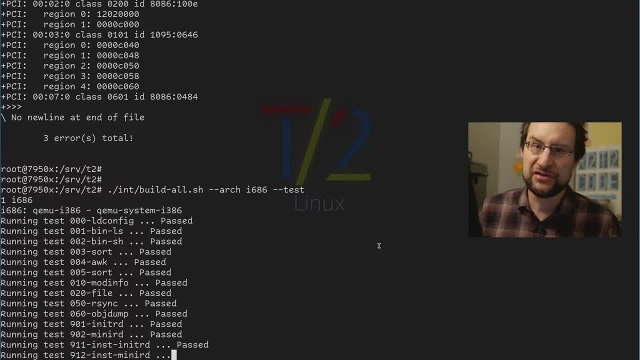 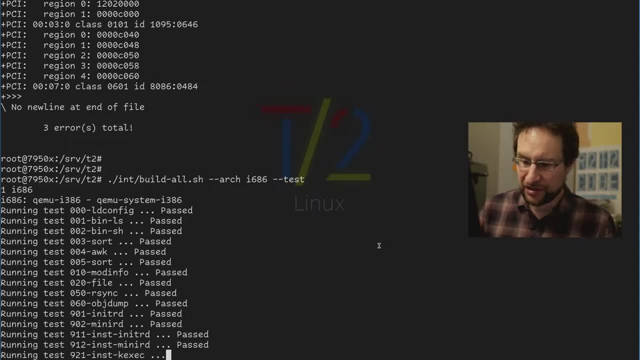 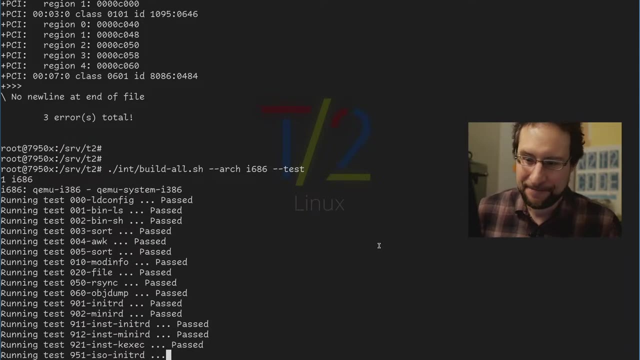 And so we started with running all the binaries as much as we can in the testing, all the freshly cross-compiled stuff through QEMU. We've done this previously and now we expanded this to whole ISO booting And of course it spent another over three. 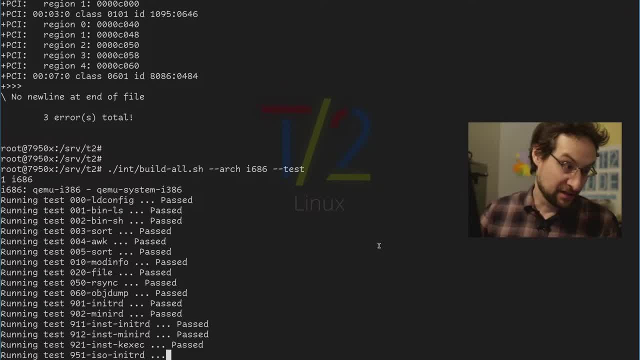 if not four hours on this stuff, fixing some bugs in between- And of course, as usual, we instantly found some bug right. I nearly would have released this release, potentially with some ISO not booting. That's also what the unit test for, right. 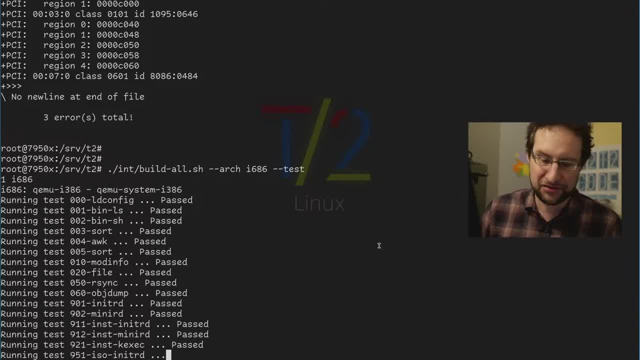 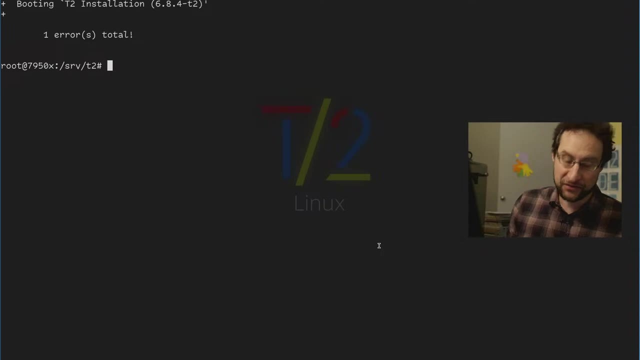 And obviously that is all this like multiple orders of magnitude faster than writing that to not the floppy, but some precious CD, right? And it's like, obviously, if we- oops, this was a wrong one, If you would write this to a nice looking CD. 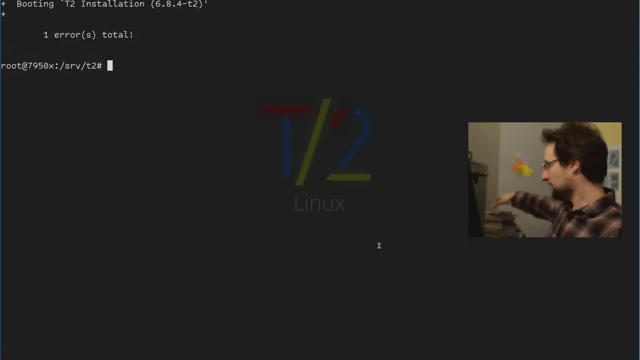 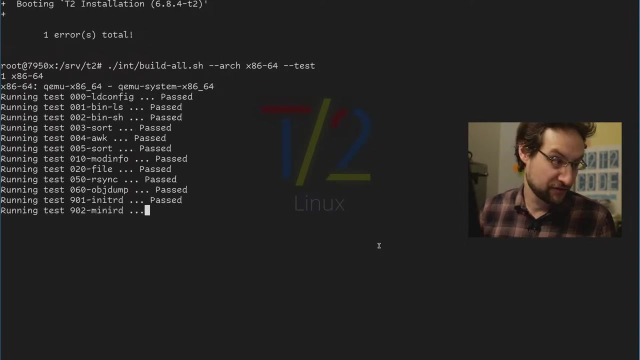 we would spend here all day Now writing CDs and manually putting that into some devices and that unfortunately somehow did not yet boot. Why did this not? So what is new is- and also welcome to this live stream- right, Working live on making the open source world more tested. 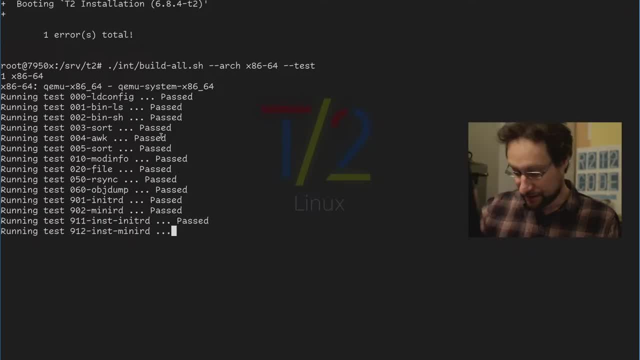 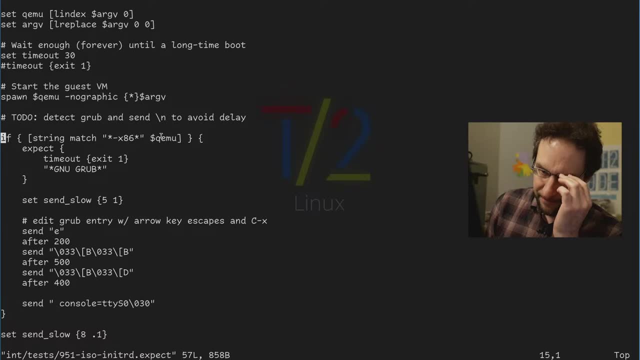 So most of the tests pass. What is new now is that booting the whole CD that is a little bit error prone. as you see, I still worked another hour on this after the live stream. So for this we unfortunately, like some, would boot. 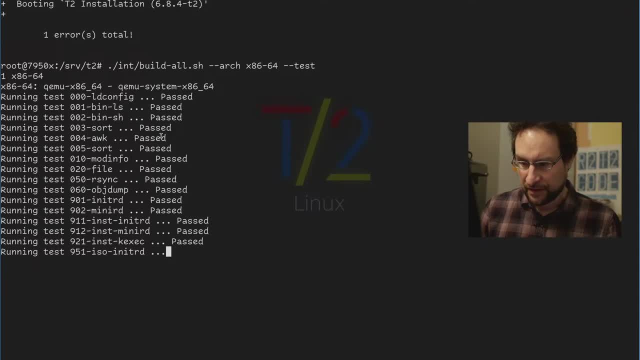 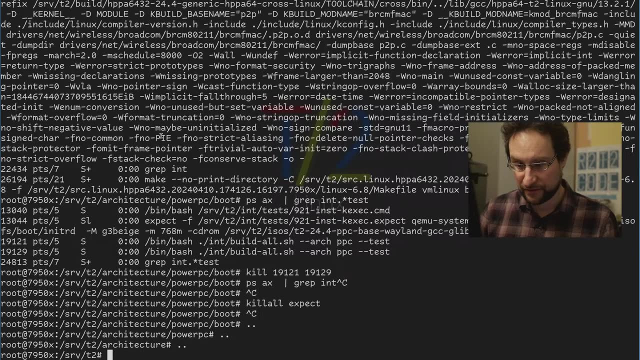 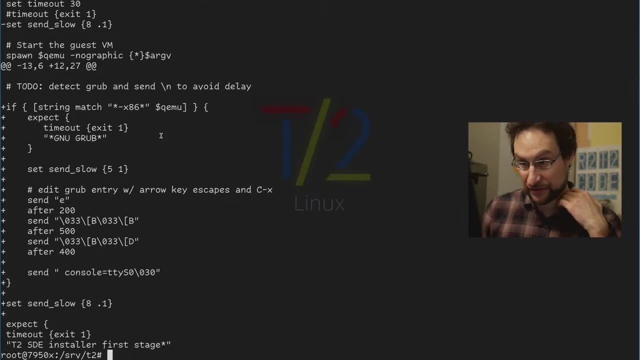 but for x86, we would need that stuff here And to show you that better, let's kill all this. expect stuff maybe away. Maybe I should also actually commit this before I break it again, because it is some fragile stuff that's not yet amazing. 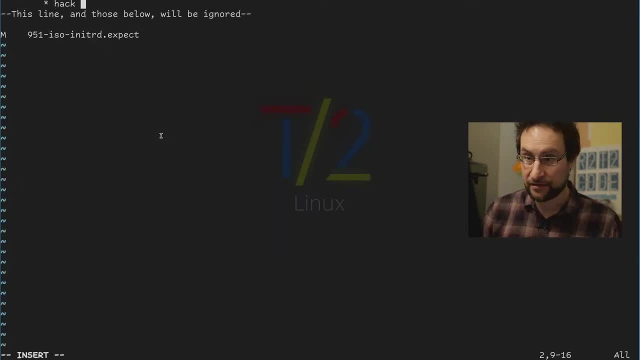 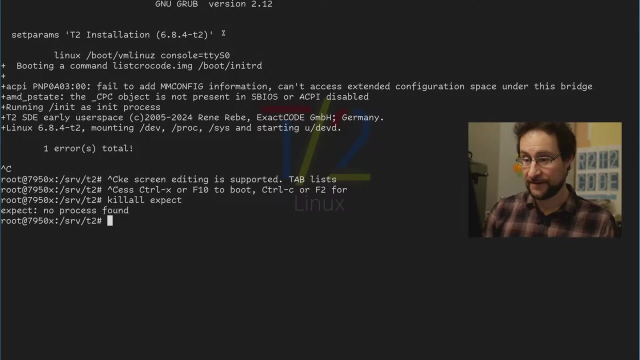 Basically commit heck X86, this is test, number 151 also in it- or the x86 to console. Otherwise it's like all other architectures gets us automatically except x86.. So to show you what's going on, so, and maybe even make it live a little bit better, 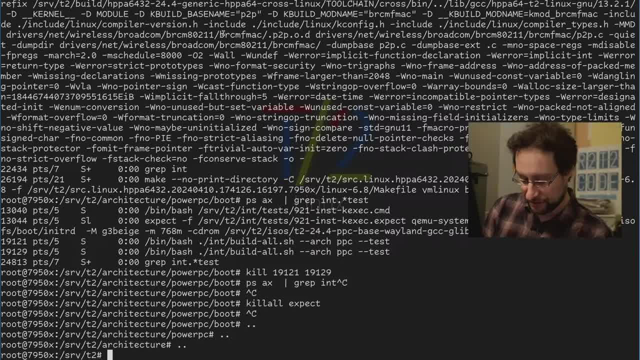 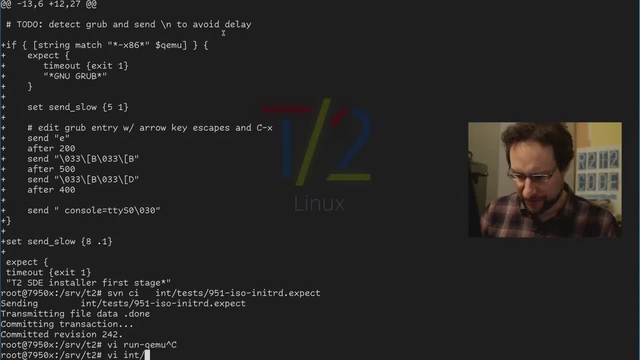 Greetings To Hamburg, Hamburg in Germany or somewhere else. Otherwise greetings from Berlin, Hamburg in Germany, one United States or wherever. They also have nice Hamburg, So that. so as I need some argument for test suite stuff, So that would be tests here. 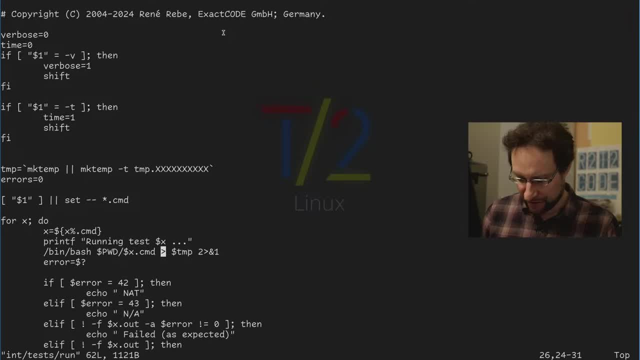 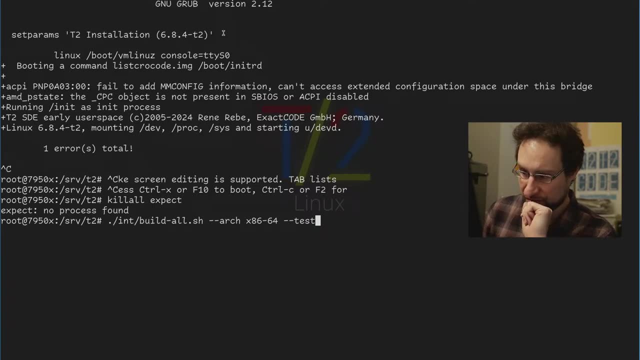 And let's, for the sake of demonstrations- only I do this while developing- to instantly see that. So that would be 6a6 dash. So we only want one test, So that would be 951 iso. So actually this did work. 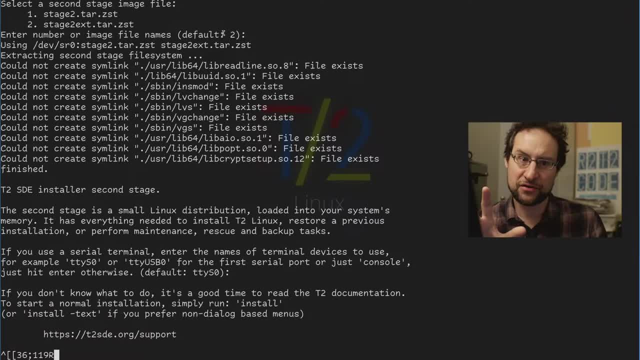 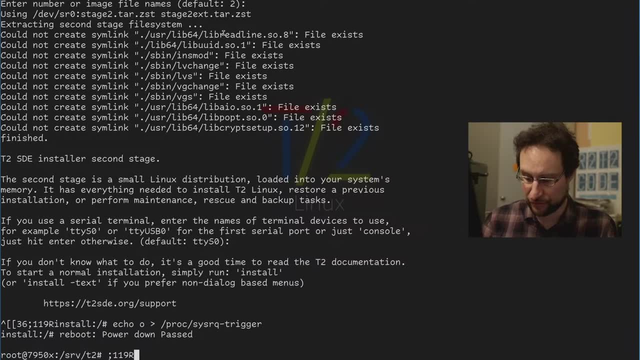 So, yeah, there's still a bit now. So this runs this through the hook here: most of our freshly produced binary, And then the test pass. it's amazing. Still wonder where this escape stuff comes. Maybe this is some strange bootloader. 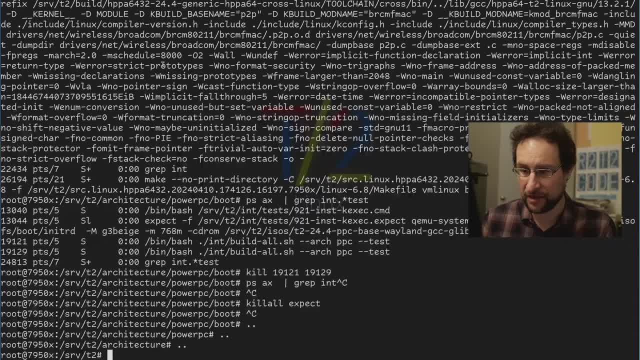 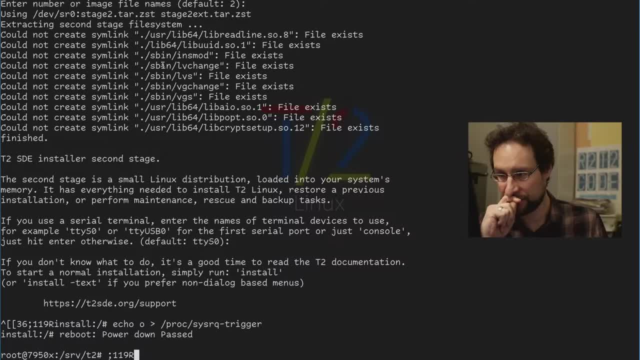 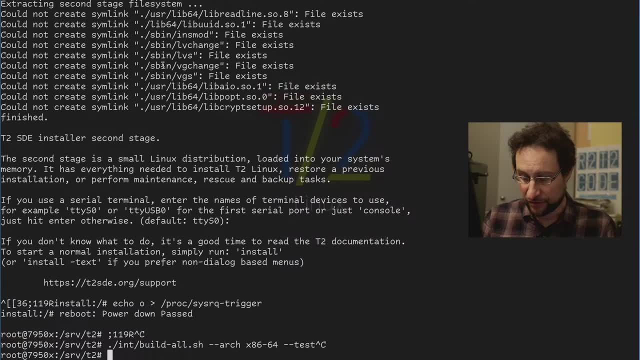 Maybe this is some strange bootloader Or putting escape stuff, So getting there was a little bit fragile. I wonder if we can improve this a little bit. And so this already uncovered actually power PC not being set up correctly anymore. I also slightly okay. 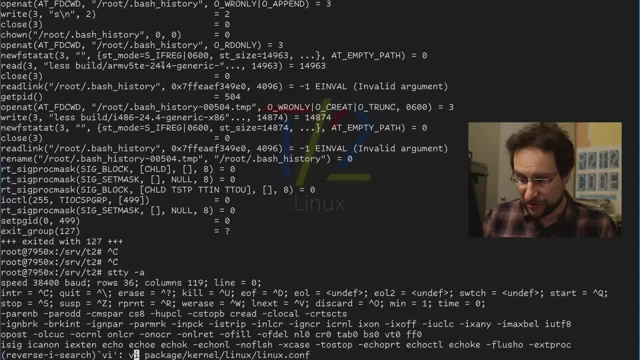 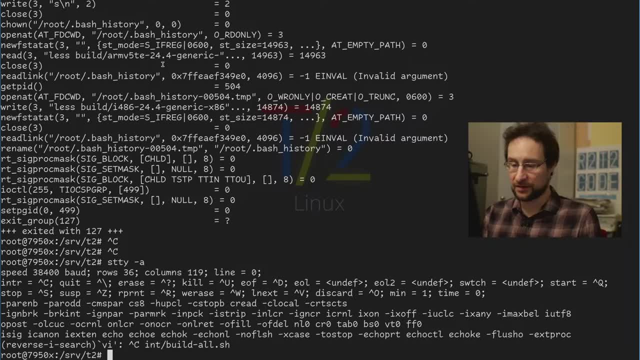 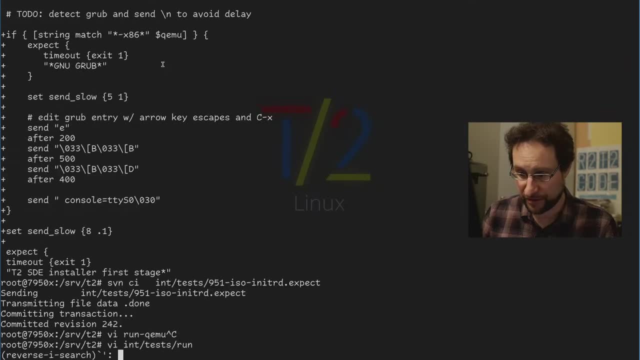 Maybe, if I do later, not to mix everything. So this was a little bit tricky because grub is so slow and characters get lost it. So this took, and I mean what should have just worked was way too much of trial and error to. this is a test like 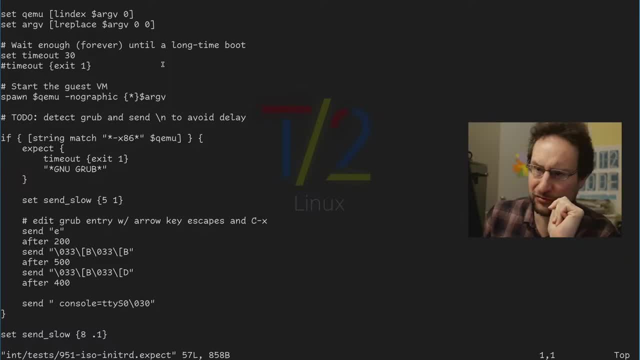 It's a good old fashioned like if you have a better like. sure, modern people do this in Python, but I would argue maybe this TCL tickle expect stuff is potentially more readable in Python, So I wonder if it can get a way. 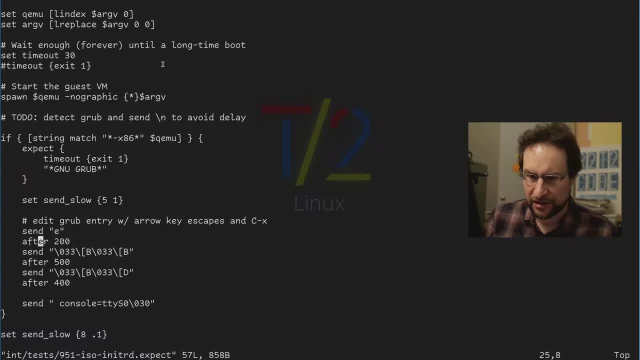 This is after, so after it's like basically sleep, it is what it is. So we for x86 we do this extra stuff. otherwise we can just like kernel will figure out serial console automatically, except for x86.. So this here is pure delay, and I wonder if we can somehow 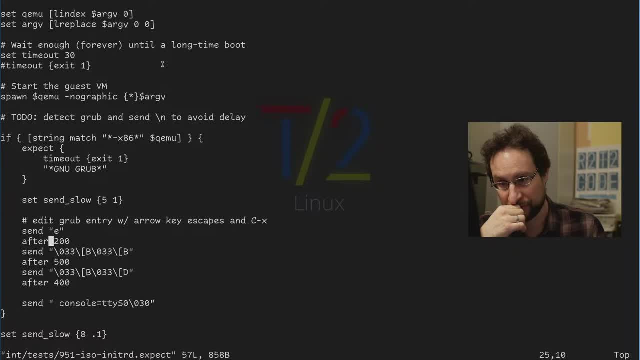 So here we already wait for gnugrap, just because it might take a second for this to. Otherwise, we send all this stuff and it's getting lost in serial buffers and flushes and whatnot. So the send slow also does not. apparently it works the most amazing. 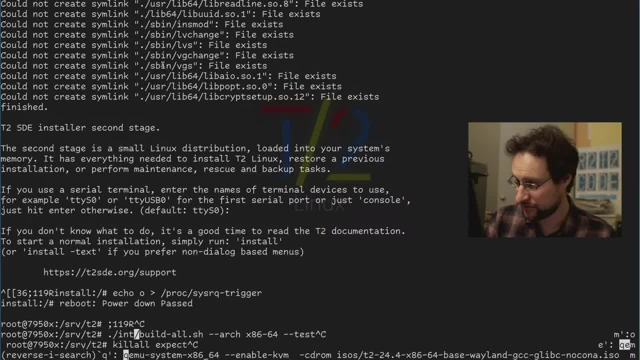 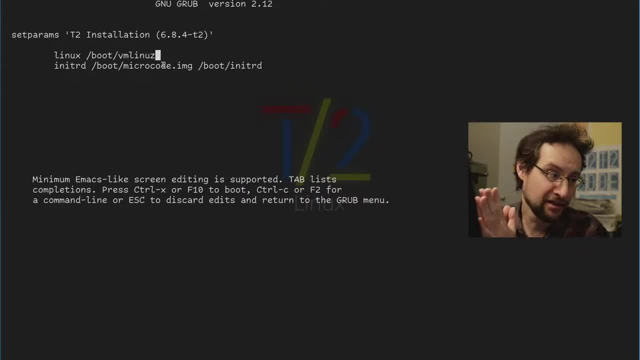 So what I do here is I edit the serial console thing in here. It's basically E, arrow down, arrow down. It's like this: Like yeah, I also would not want to do it like that. I ideally would want to grub or something, autodetect the EFI or whatnot- serial console. but it is what it is right. 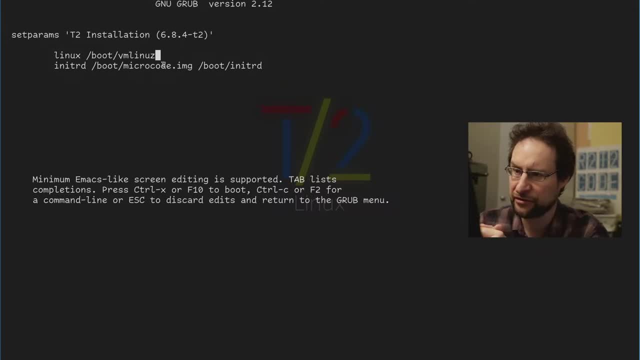 You gotta do what you gotta do. I mean we want to test this stuff today. I don't want to make a week-long research project of how to autodetect. I mean I googled and like even Google or ChatGPT doesn't have a solution for that. 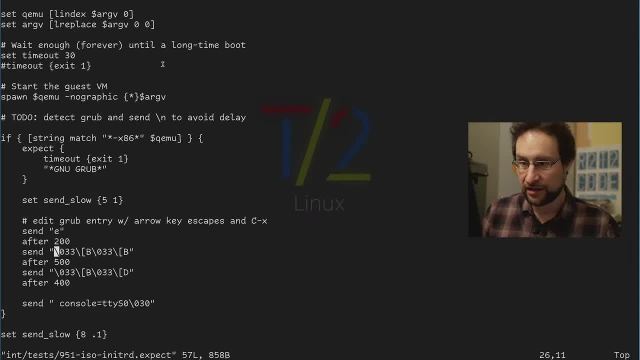 And then editing the stuff in here, right, And then sending. so what this stuff is? it's escape codes for So E down, down, like wait shortly. I wonder Basically what I would want to do is: can we get away with some of this stuff, because it's just freaking annoying. 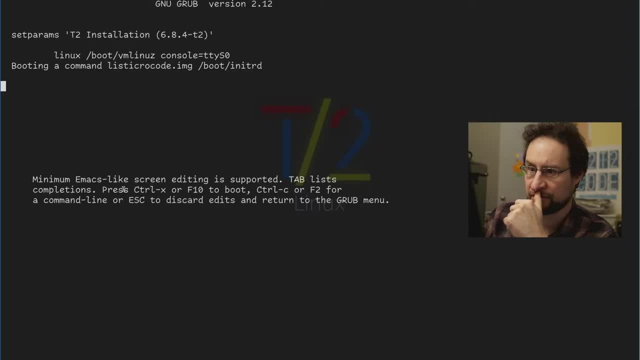 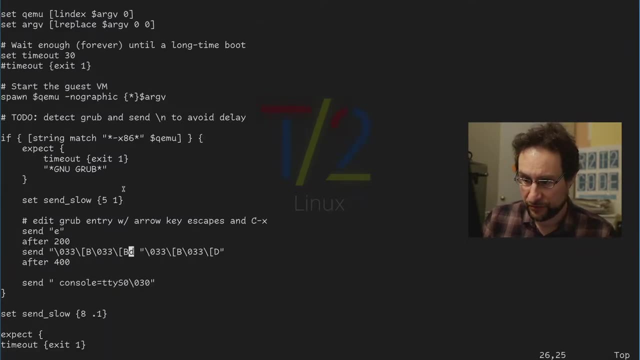 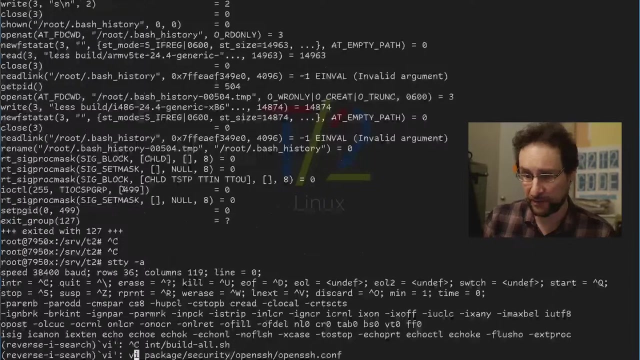 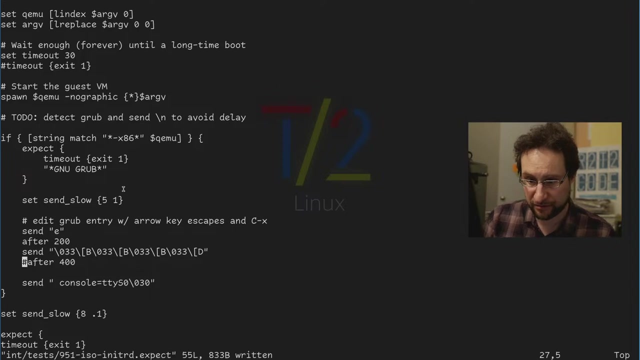 And so that is that. Okay, that currently works. So let's unify that. Does it sense to? because I this did not previously work. Maybe the after thing fixed it mostly, Because you will see that. Okay, let's comment it out. 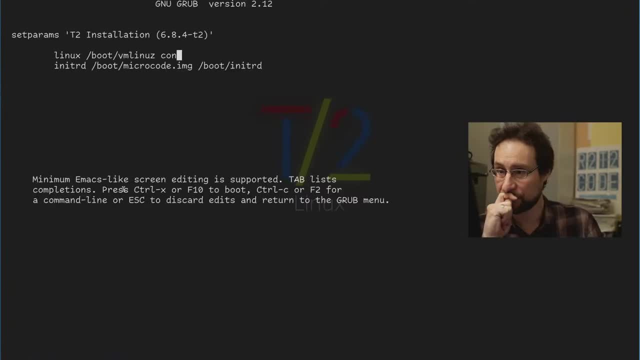 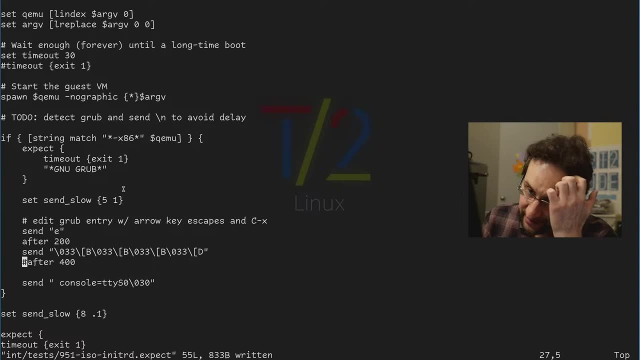 Does this still work? Yeah, so this does not work, right? This is why I ended up like I was like half an hour, was like: why does this stuff disappear? I also wonder if maybe, Um, Because I have to send slow stuff here and I still wonder. 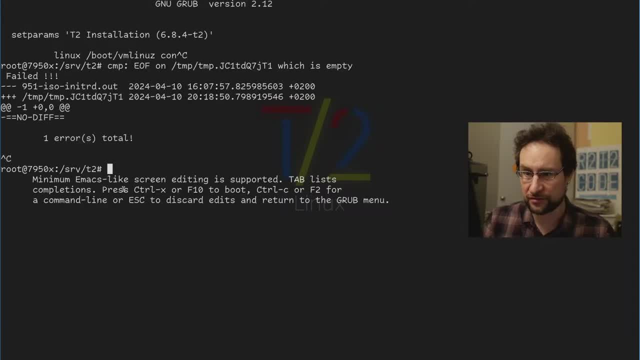 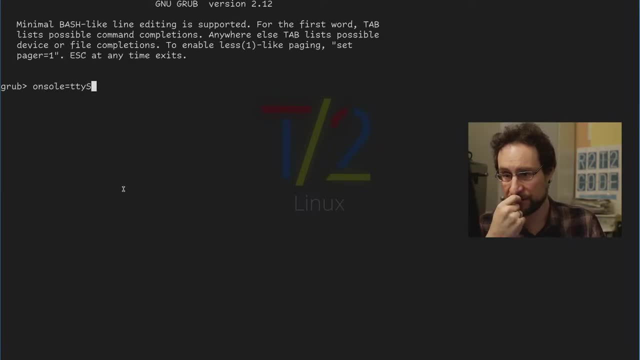 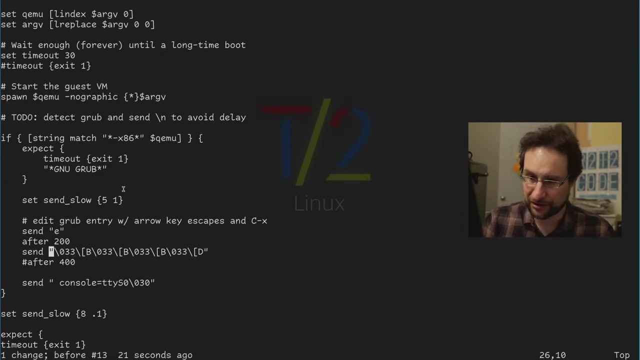 Apparently, we might need to use Uh S, But I also didn't have like okay, so I didn't have the biggest Oh wait, this is also not. So yeah, I'm This. this totally sucks, right. 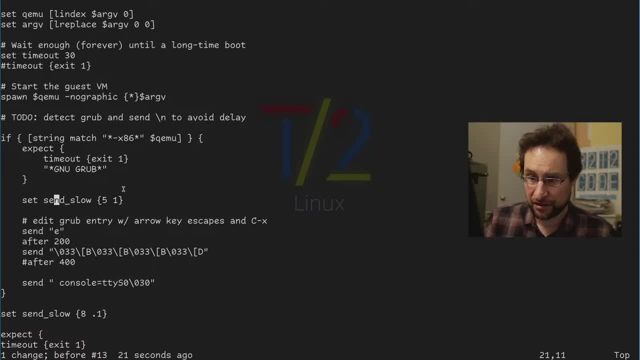 Like: this is the most, one of the most annoying things here. So this is I mean, maybe this is too slow. actually I wonder if we like So also this editing, like: if we run this manually, you will see that, like it just. 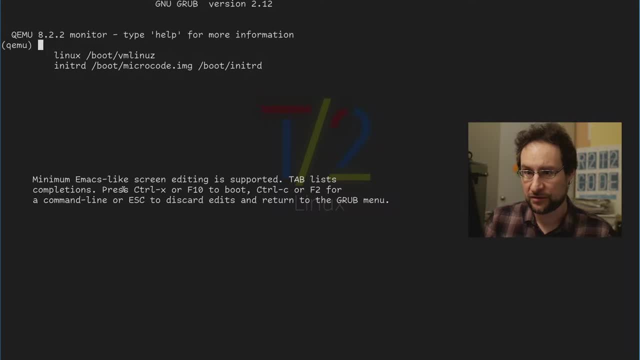 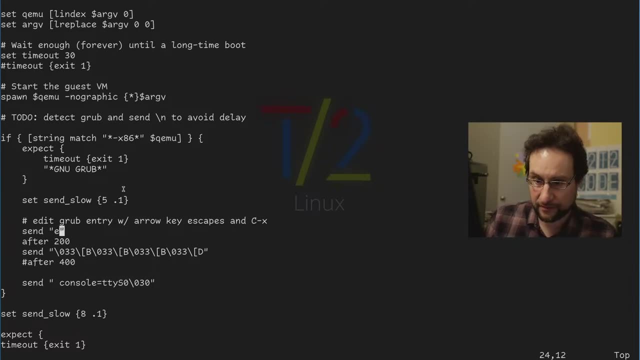 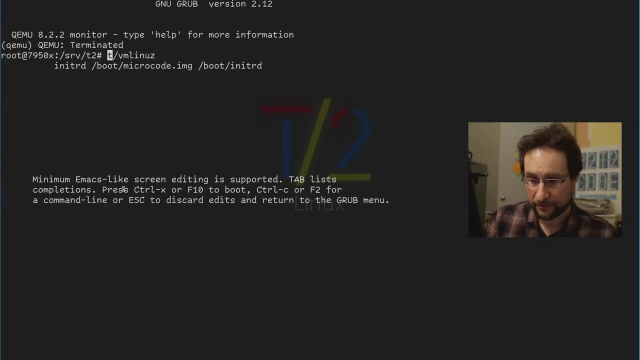 I mean, it wasn't even that slow. but So the question is in. Yeah, Basically, the question is: what do we need here? What did I even? So? this is, of course, super error-prone, right. 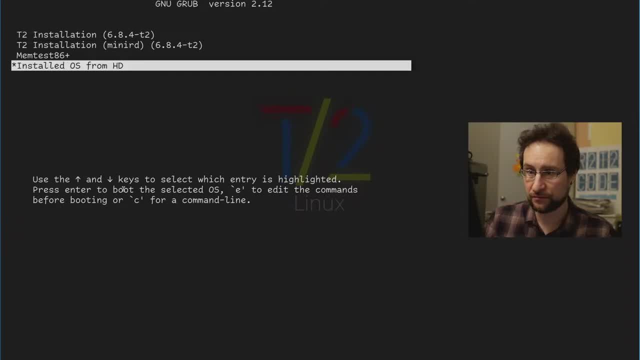 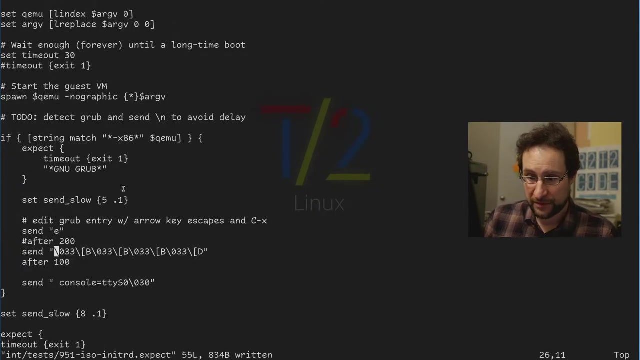 So this is, of course, not how we do reliable reproducible. Uh hello, What did I Do here? Okay, that works. That's basically speeding this up a little bit And making it less Like. basically, I spent already half an hour to get even to that. 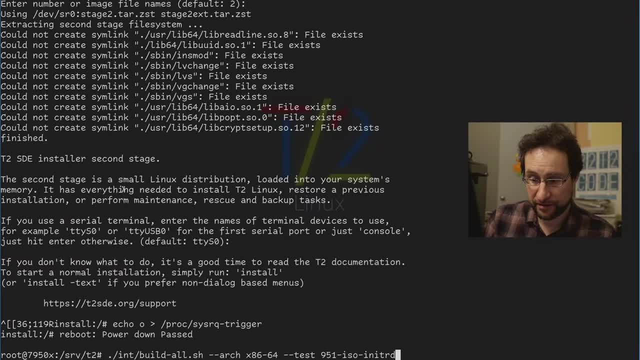 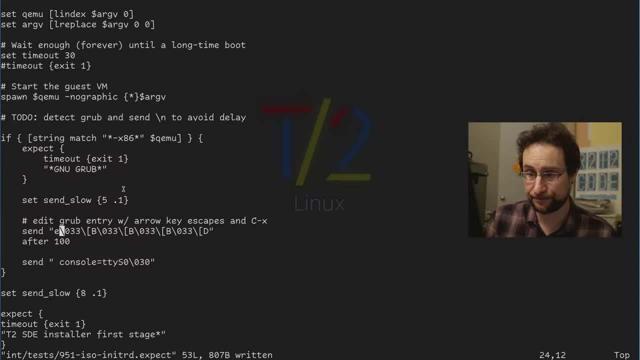 Um, The- I mean initially I had it all in one line and it didn't work, and I debugged it forever. Is that, crazily enough, also still works? Um, What do we have now? Okay, maybe this other one was even too slow. 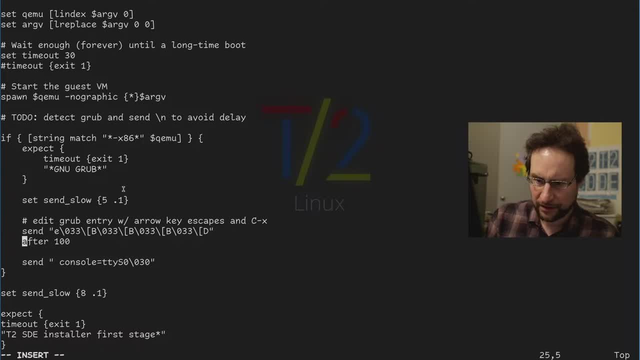 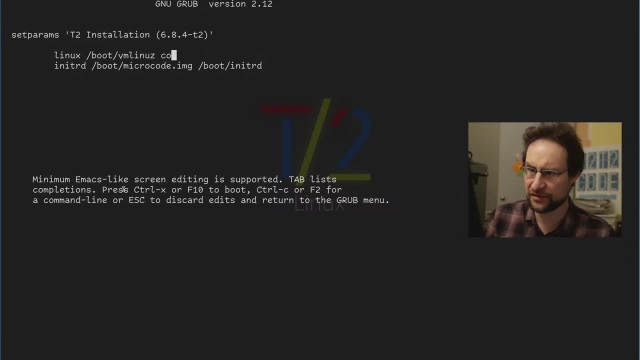 Maybe it doesn't. I wonder then if that works combined way. No, it does not. So like there, you see how error-prone this is. Um, I also wish it weren't like this, but like I didn't write all the software, 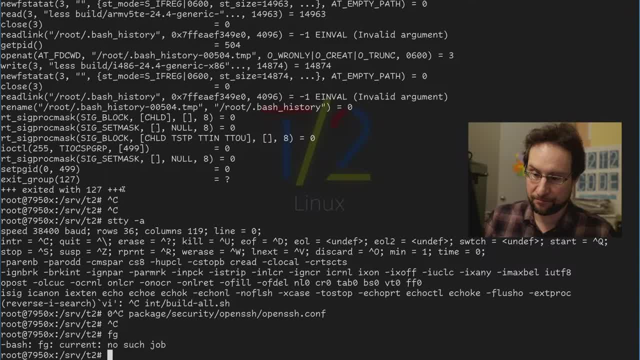 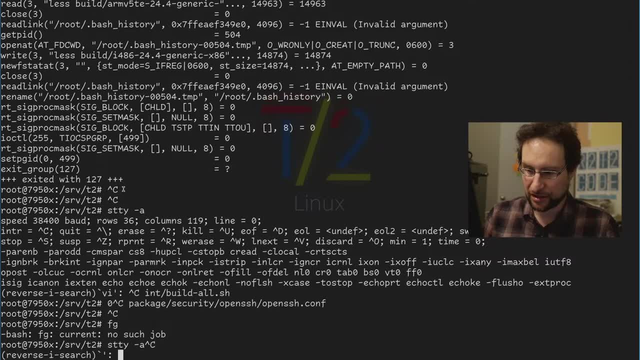 And it's maybe also explains why many other people I mean it's like: yeah, I mean even testing, right, It's always. People are always surprised that test engineers also get some salary. I mean, obviously you also need to live. 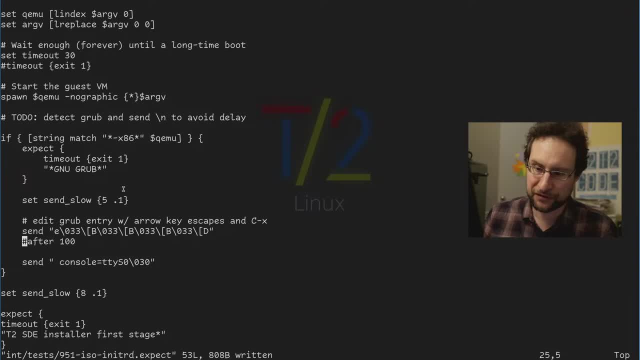 Like this, All those tests you Like, the handful of tests you already took, like basically easily a 40-hour week of just scripting all of this stuff here. Um, All right, I mean, maybe we could actually watch here with this stuff. how slow this. 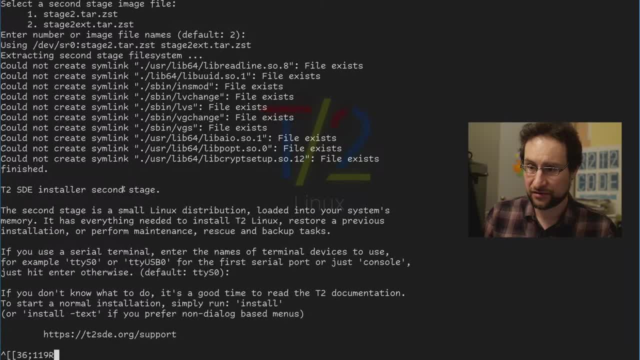 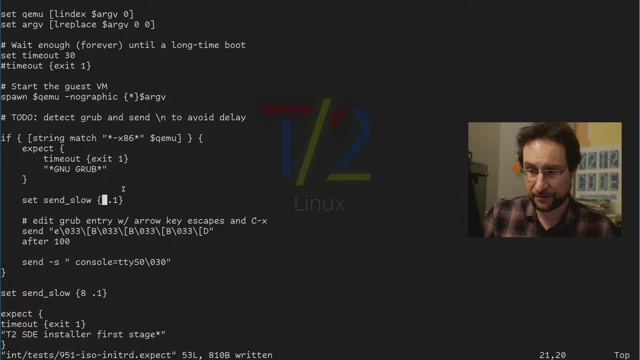 Because the documentation says this is also, But this is a little bit fastish for my taste of Does this even have a proper effect? Oh wait, This is actually a .1 delay after I mean, let's make it super slow or somewhat slow. 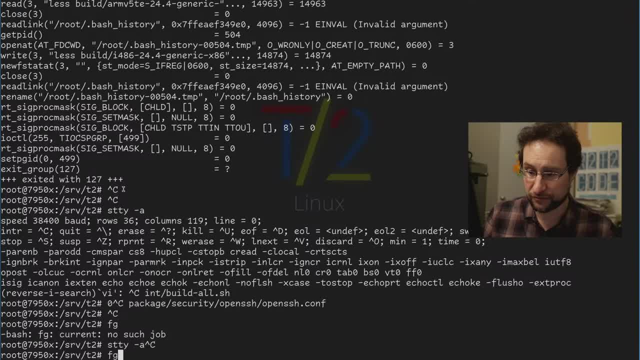 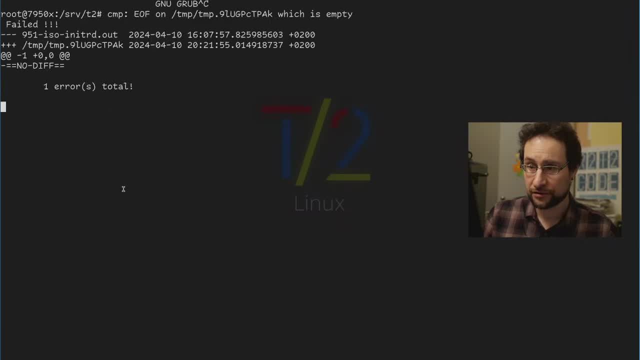 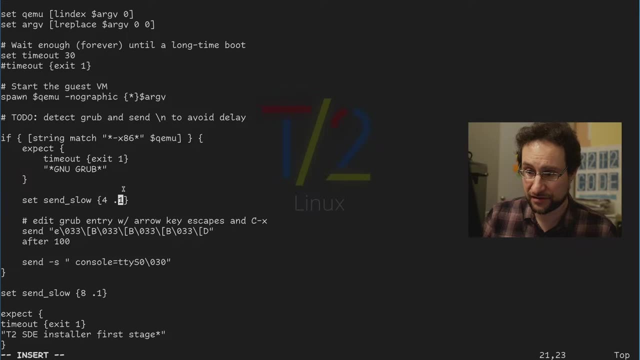 So this should be after every two characters, one second delay. Can we watch it like: Okay, this didn't work, Okay, actually. Okay, this is actually making this here maybe too slow. Okay, this did work with that right. 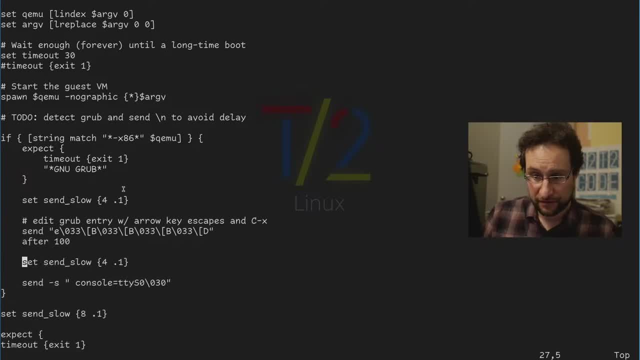 Let's maybe analyze if we make this here really slow. I mean maybe the bloody escape code somewhere may I mean on a real terminal. they also should not be that far apart. I mean, maybe then breaking a pair of four breaks is. 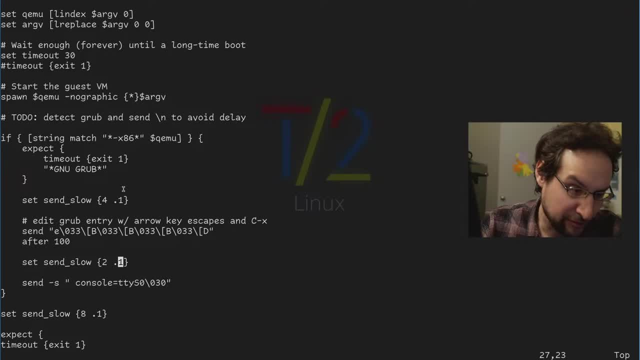 It's like, yeah, maybe people have better ideas. Welcome everyone, By the way, do we have zero frames and audio? That's amazing. Manila greetings there too. Early morning here. Happy that you can tune in and enjoy. 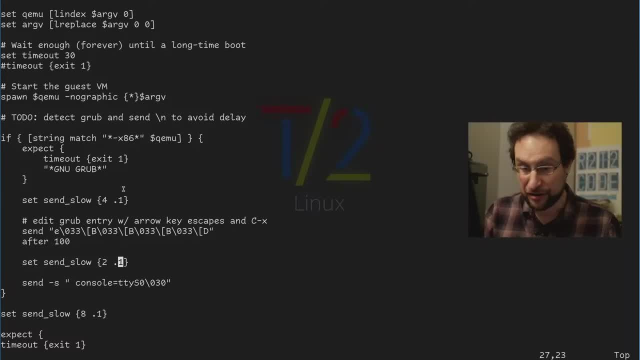 And I hope you learned something, especially how not to break your poor PC. We don't even know how this iBook break right. Like I tested so much, nothing tricked here- Absolutely mind-blowingly crazy stuff. So let's try this again, if we can. finally. 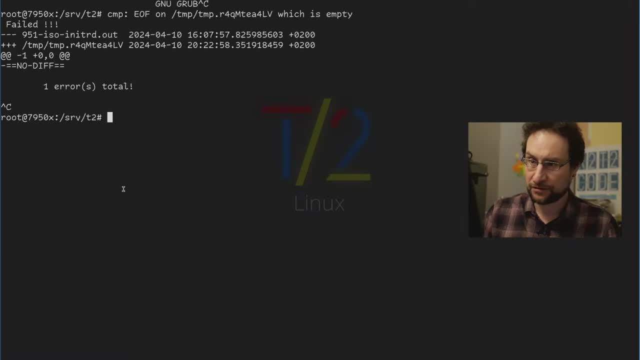 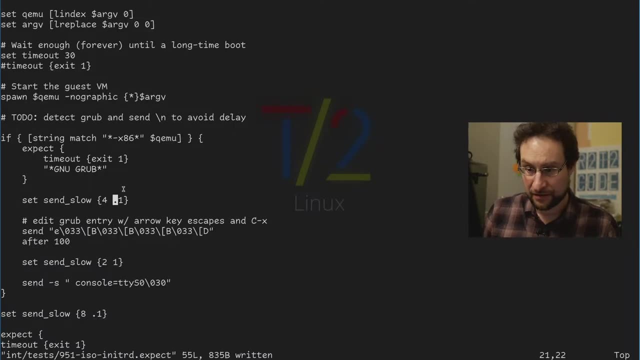 This is still not like work. What's even going on here Like this is why, like Half an hour I only spent on this mess Every 4.1? Like, like. what's even going on here? 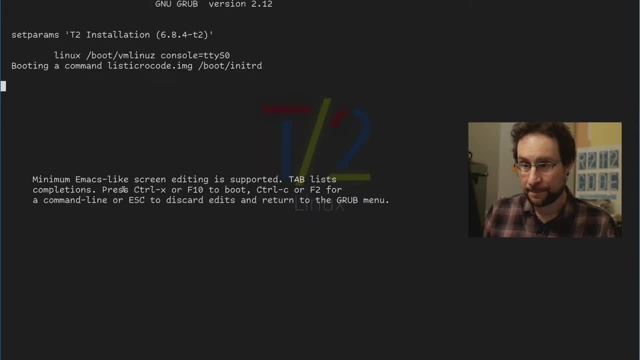 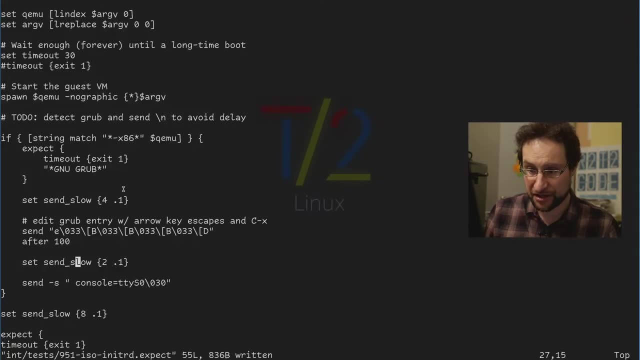 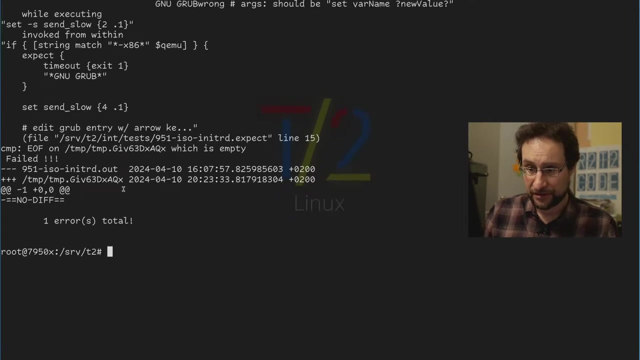 I don't. I don't even quite understand, And what I also. The documentation theoretically says "-s". I'm, I'm confused. Does this kind of slow stuff in all the tests even work Or not? This is What. 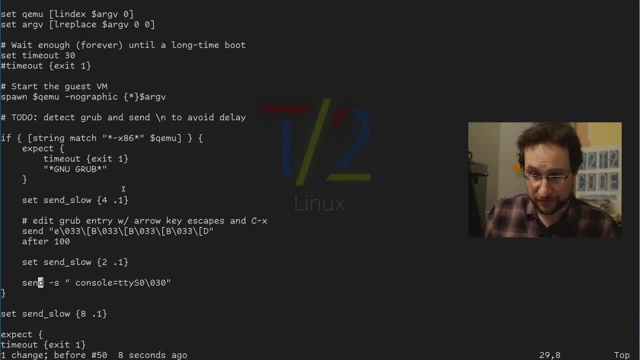 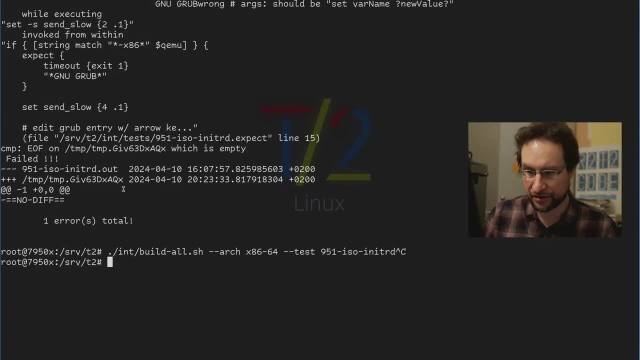 Wait what I don't know? Ah, set, This is so wrong. Ah, I had here "-s". I mean, maybe this is not even sending slow And "-s will break it again if it's too slow. I mean, it clearly has some effect. 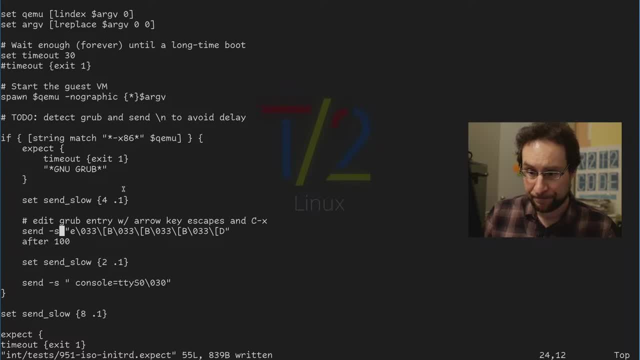 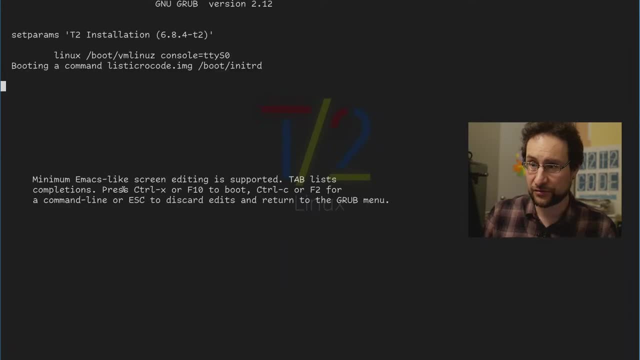 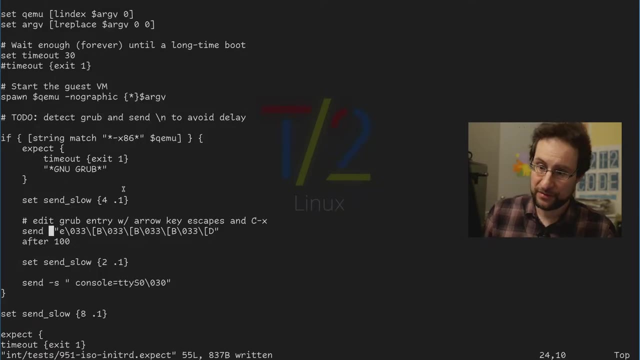 Just not the most desired one, But maybe, Maybe this escapes stuff, I mean it's. I mean, of course it totally sucks that this is so, Um Yeah, Unreliable, But I mean, at least this works. 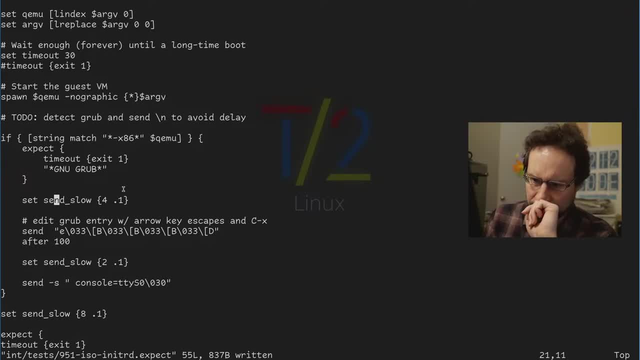 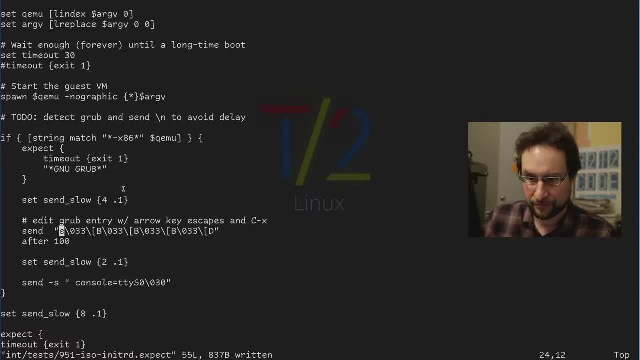 One, two, three. Um, I wonder if those are in. Did I have to Extract space here? I mean, yeah, This is not the most rocket science thing, right? Um, So what? What was it? One, two? 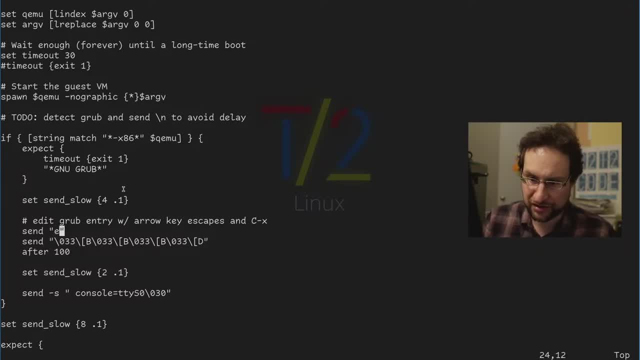 So it's Like after every three, like one. does this like work reliably? Nah, And I also wonder if we need this delay there. Currently, that works Okay, Okay, Okay, Okay, Okay. 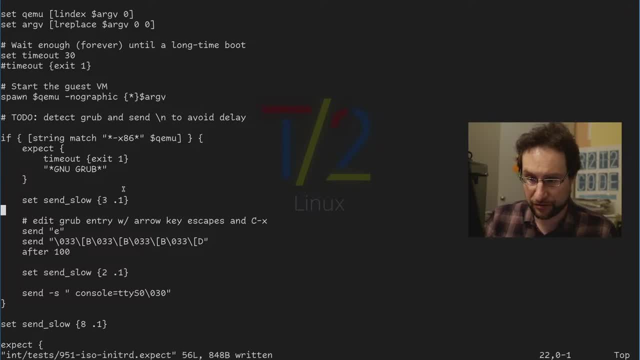 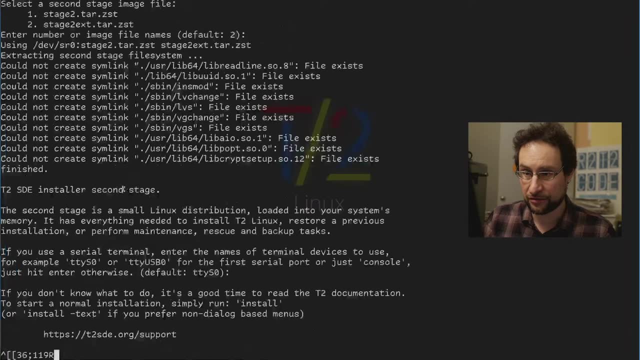 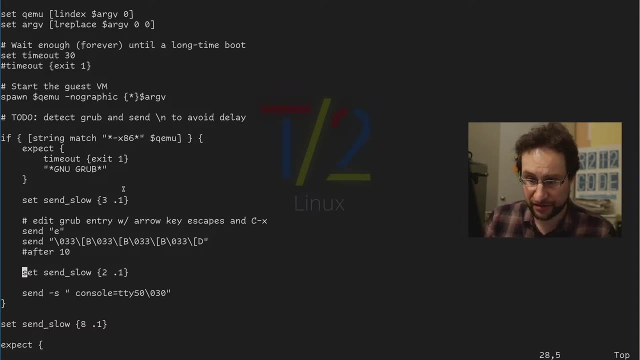 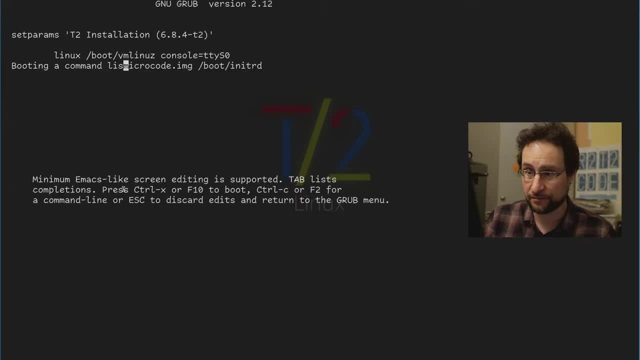 I mean: do we, Do we even need that then? And so this is This. we send slow right. So this is apparently S. I mean this currently works, and the question is like how many others? 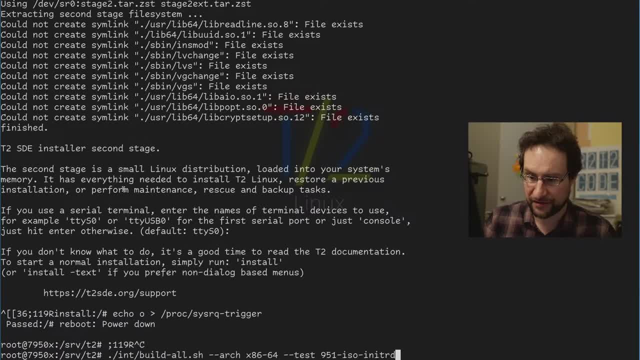 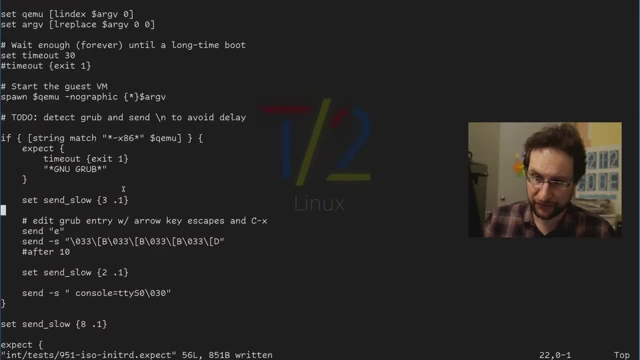 So send slowly Here. we don't have "-s" right. But the question is: Apparently also works And like maybe this pair of three here was not like sufficient Okay, Okay, like four, one, two, three, one, two, three, one two. 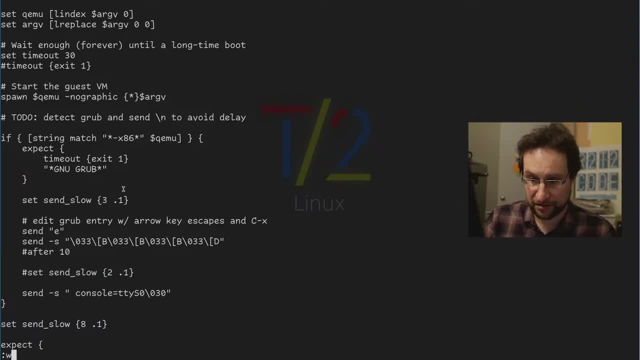 I mean yeah again, I also wish I wouldn't need to do that like that. it is what it is, Cause it currently appears to work quite reliable. I mean I guess then we can delete all. I mean we could leave this in as not to. 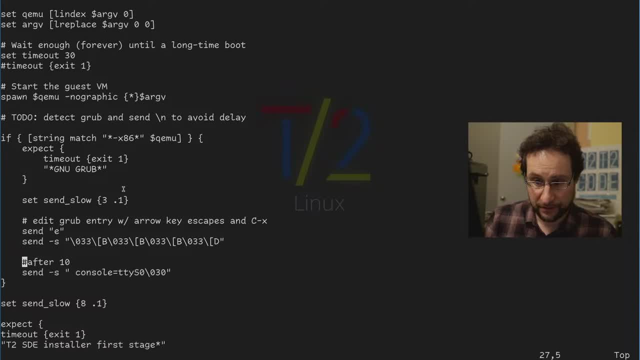 like basically as a reminder how to do that, in case we need it again. I mean, okay, I'm pretty, I'm so much more satisfied than oh, this is also not slow then. So yeah, I mean, maybe that makes some more sense. 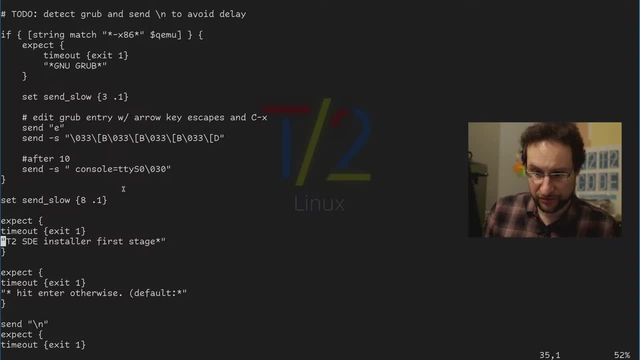 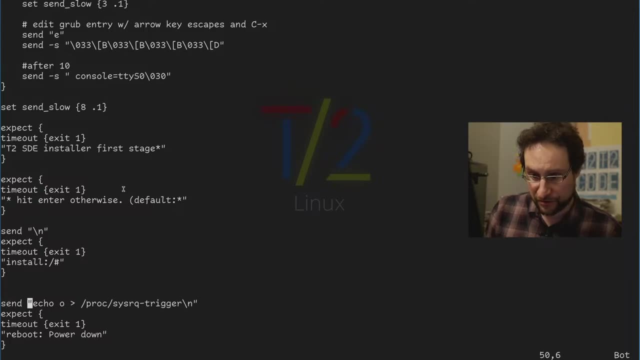 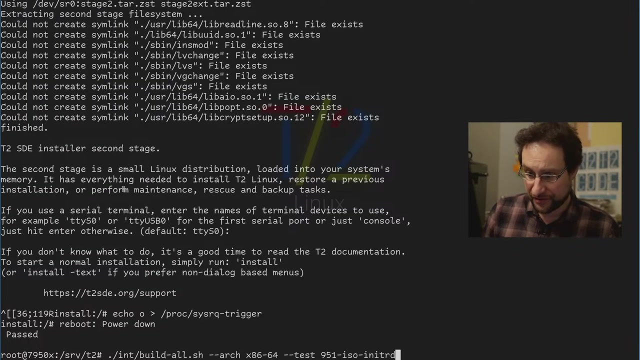 Although I have the impression that maybe this is not using, or do we actually? no, I don't. So I wonder. I mean, there are other ones apparently work, not slow, but anyway. So how this looks in practice is that we can. 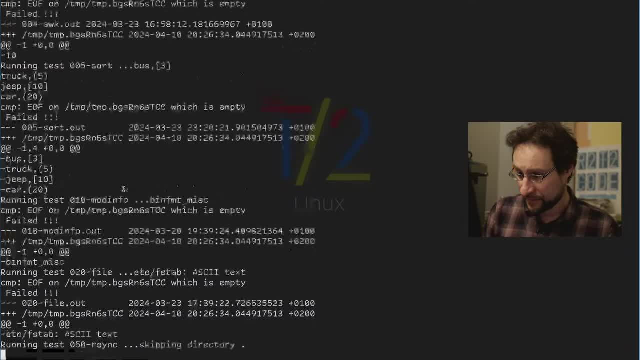 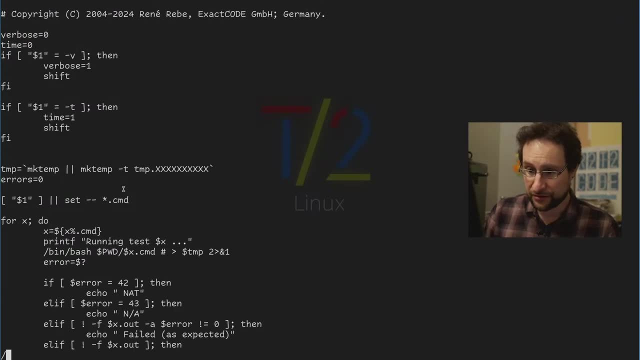 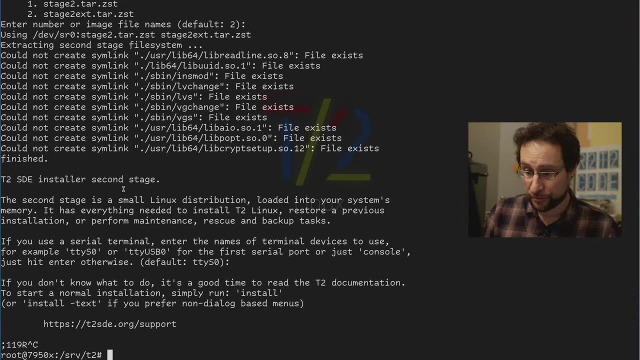 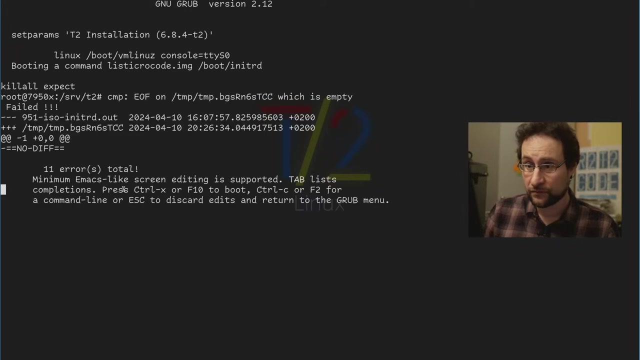 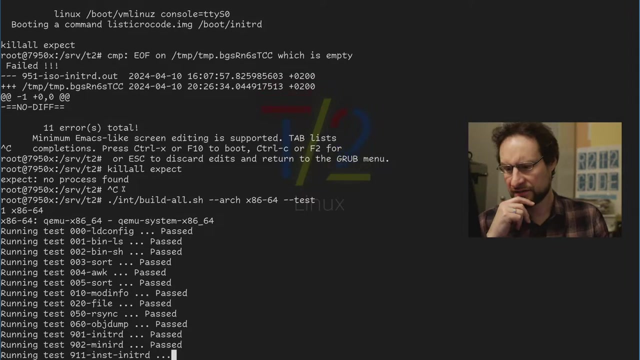 like usually it's in all tests and we have an oh, this is because I had this here. I need to work on some better way of temporary disabling this stuff, Oops. So have we killed everything? finally away, hopefully? So this is what how it looks then. 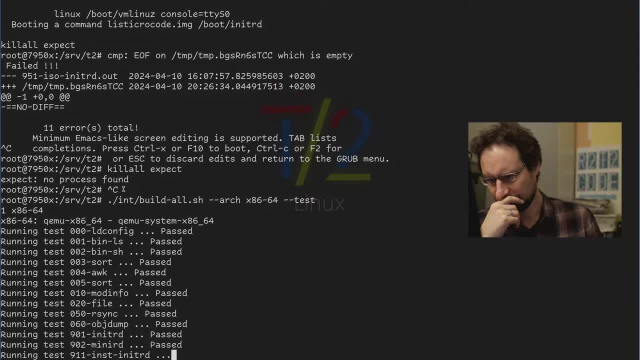 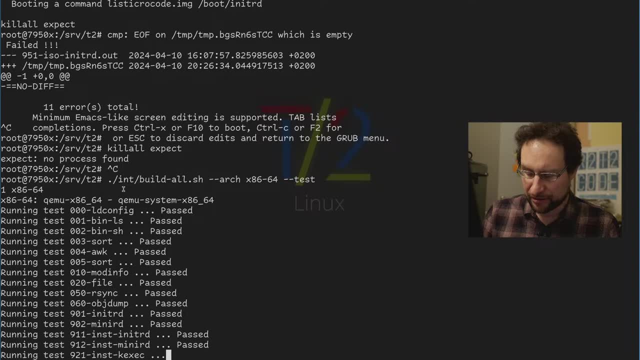 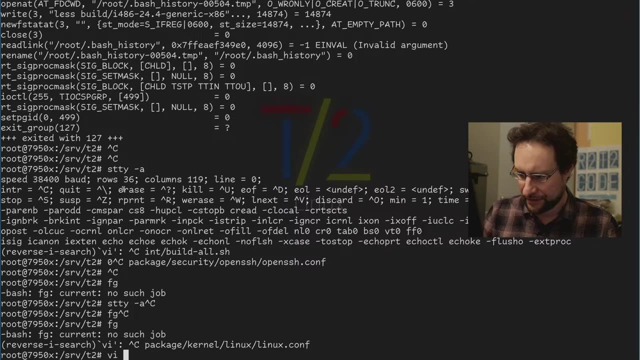 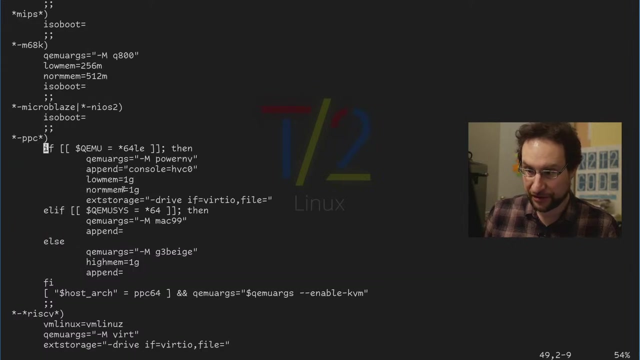 This is just a little bit of a refinement. We need one PowerPC. I still need to disable, right? So some of those tough tests take a little bit longer. Let's internal tests, QA mode, So matching here. PowerPC LE doesn't boot from CD yet. 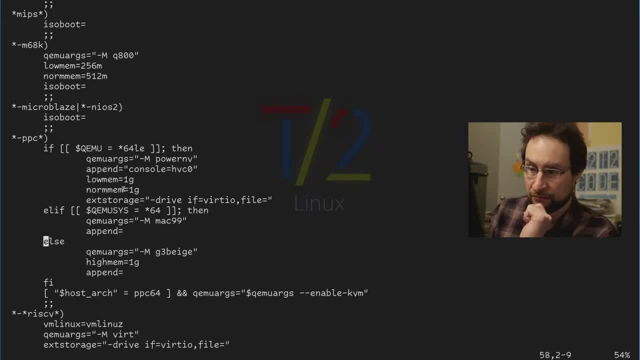 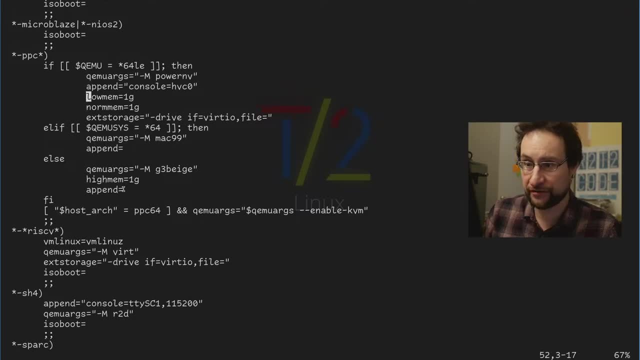 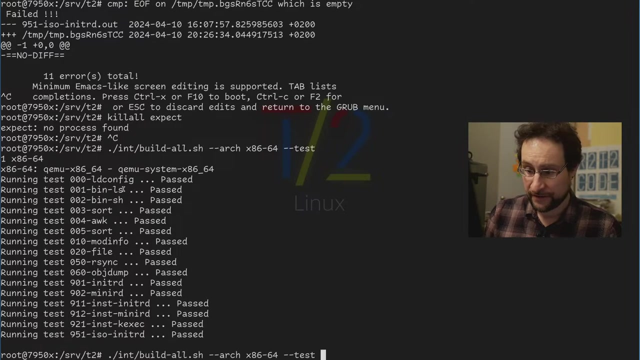 I would need to research that. what boot load or what not? Why do we have that here somewhere? 64.. Okay, here we have LE, but we can't boot this yet. So ISO boot clear that, Then we can also test all the rest. okay, 64.. 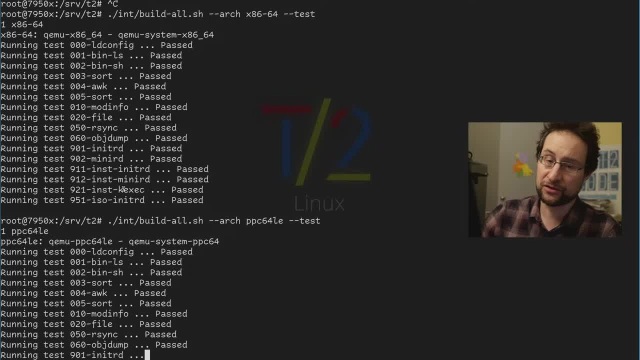 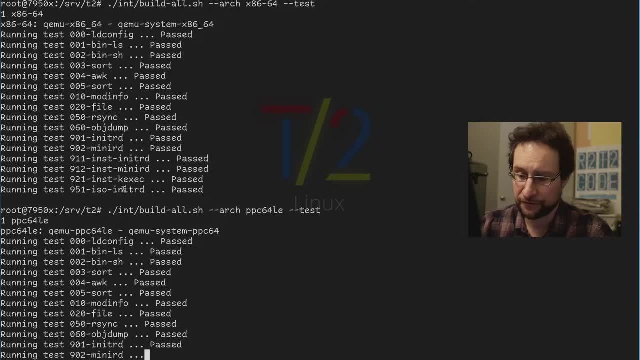 So usually this would run automatically like building the. oh, there we go. Okay, So this is the open source field, like in Epic thread, gripping cross, compiling all of those 500 or whatnot, packages of all of EXARC and Firefox and Wylent and all the other good stuff. 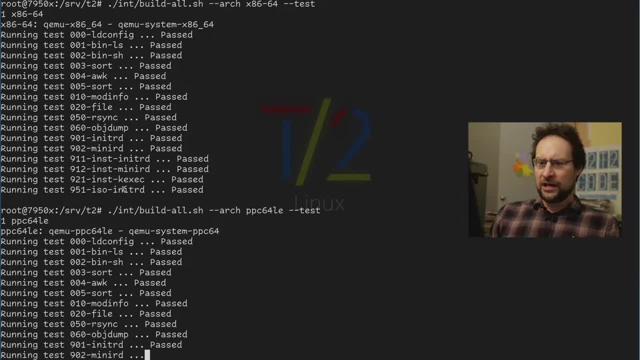 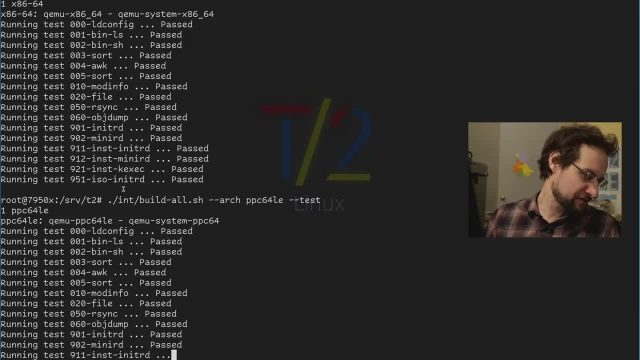 Linux kernel and grub, the applicable Testing all this stuff. I today also further refined PowerPC booting. I still need to test whether that really works on real hardware after It is possible, given that, like I booted the heck out of this. 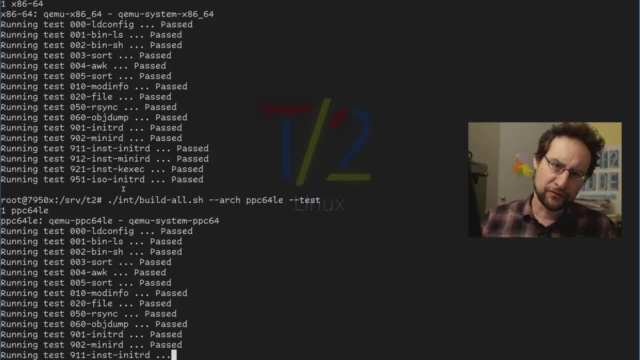 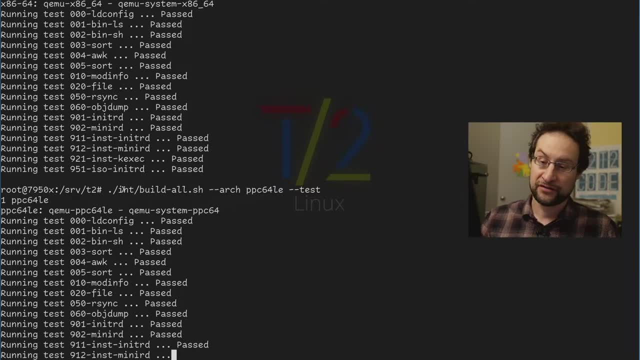 I mean, I don't quite understand, you know, I don't know, I don't quite understand why some ISO- from February I basically disabled this- moved this to defect. don't use, or so, subdirectory Boots in QEMU. I network booted similar new binaries. 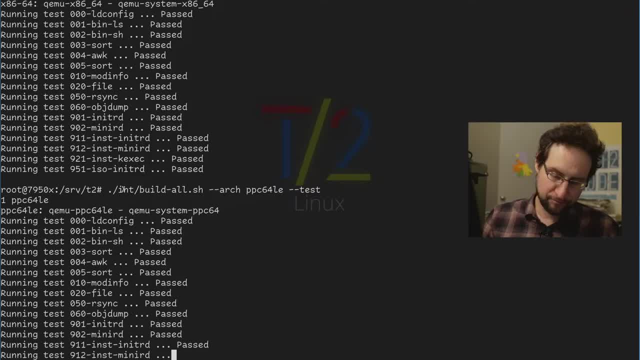 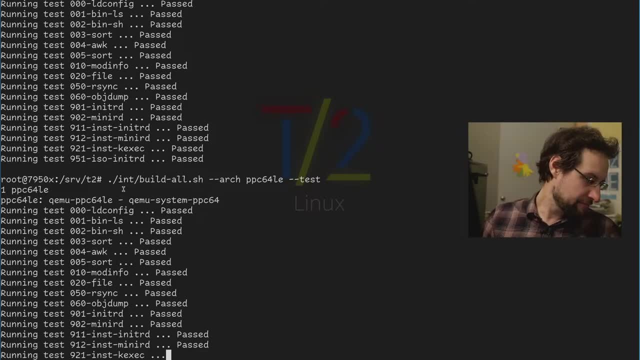 I'm not this identical, but the last days builds I booted, net booted on G4 cube, G4 Thai book, G5 XRF, Mac desktop. So why is this one ISO did this? I've like no idea. 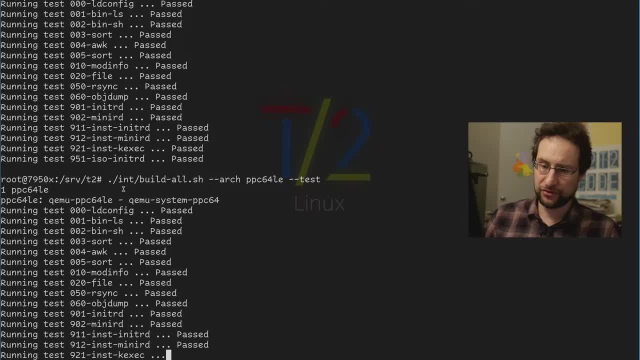 The only thing we can do is test more and unit test more. Theoretically, I would want to improve the arm build. So yeah, this stuff runs a little bit slowish. We could theoretically speed this up by running this on an XRF, which, in the long-term, maybe we would do. 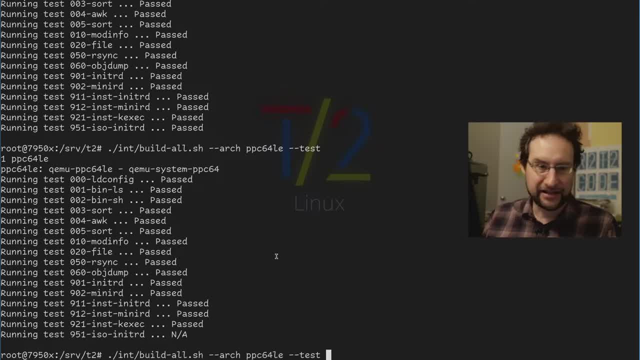 In the or okay, This is not applicable, because this was so. all the other is that like, if that is not at the end of the week. this is certainly what makes the heart beat and software developers fall in love with their right. 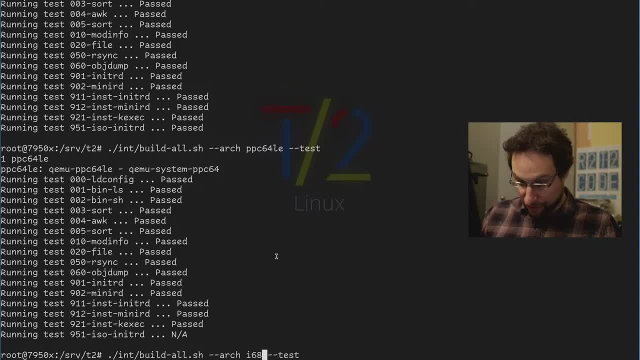 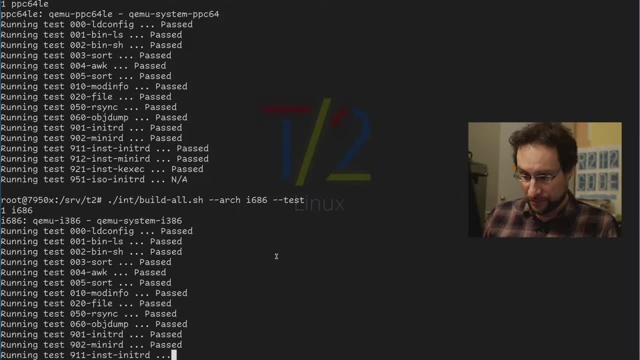 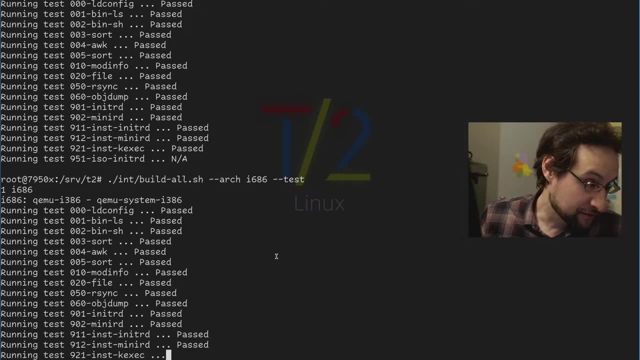 Software achievements. We could actually check x86,. does that work too? It should, so it's a little bit faster. Also running through KVM, it probably should all work And then we can. as one last thing, don't run the test for exit. previous video. 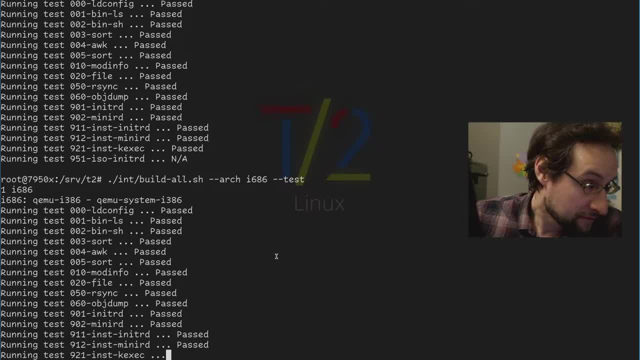 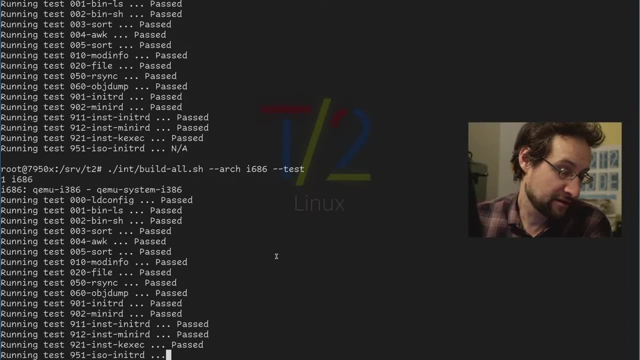 What else do we have? Why not use, expect commands that are aware of the recent text? What do you mean? I do that. Do you mean for each character? Do you mean like writing this with like 60 characters or 60 or 20 or whatnot? 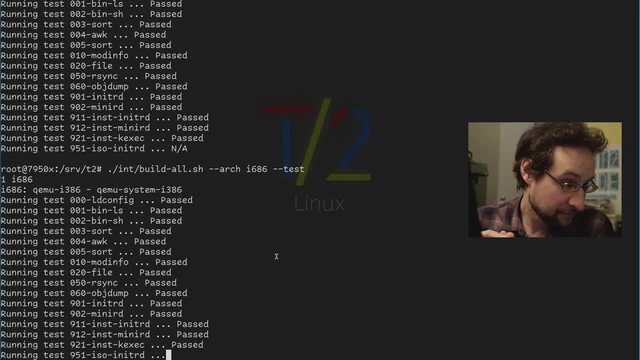 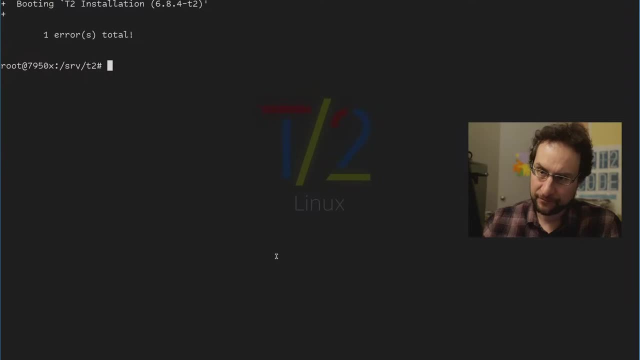 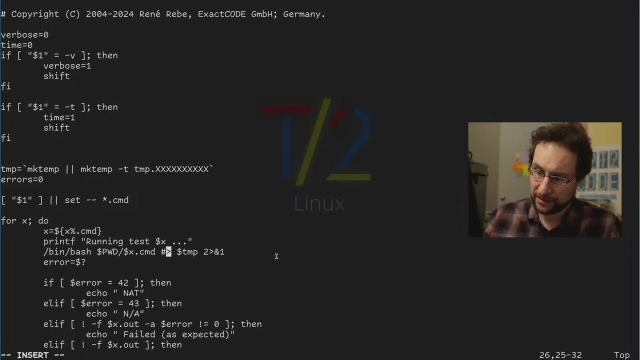 Like expect each single character we echo there, or So the question is, the 686 thing does the whole unit- I mean maybe this booting, so that didn't work for some reason. That's unfortunate. Yeah, I need tier, like I don't know what, like maybe. 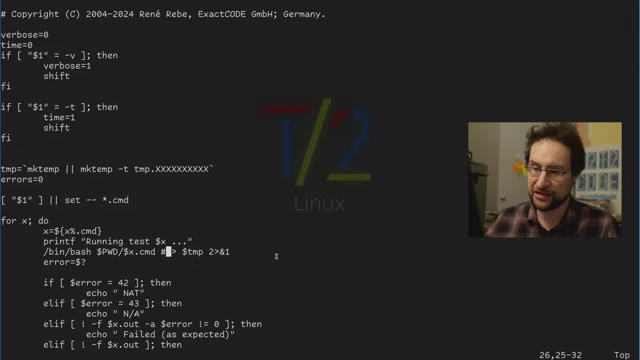 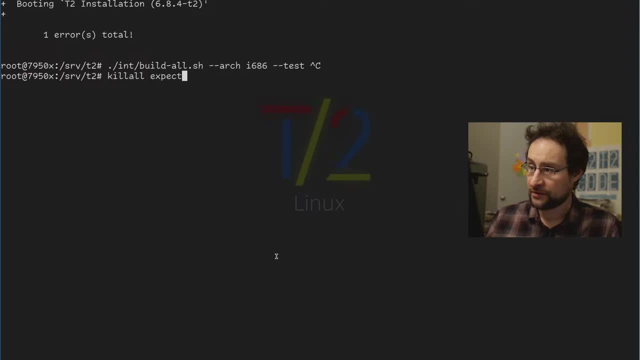 I mean this, is this already. I mean this is already. maybe I need double verbose and then teeing that to standard auto stuff. So this is, we can run selective tests right, So this would be this one. Why does this fail? 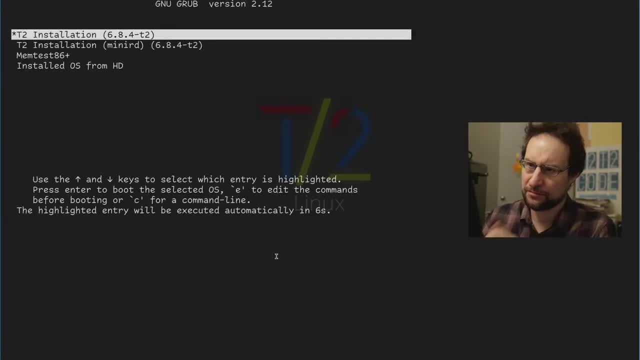 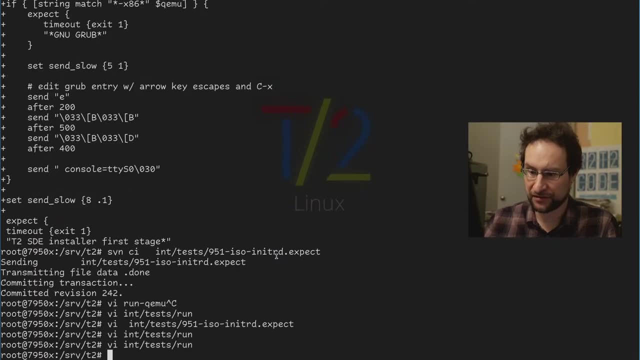 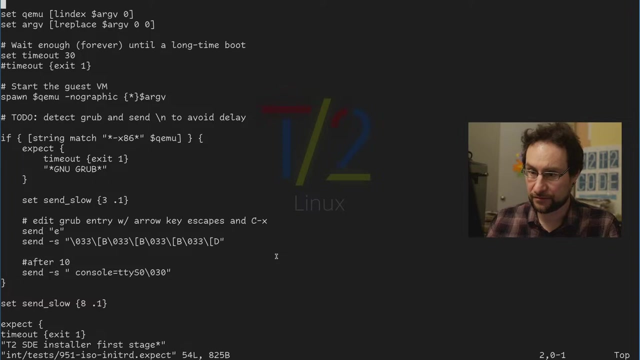 686, or ah, this is not. ah, oh, no, Ah, okay, I know what fails here. okay, So Zulu test fails because I'm matching that on x86.. And so we actually need just 86.. So either three. okay, we can dash. 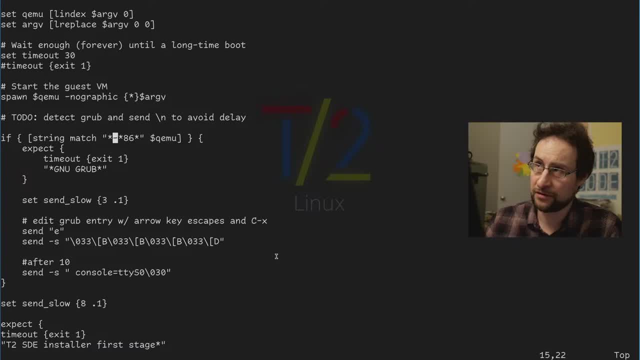 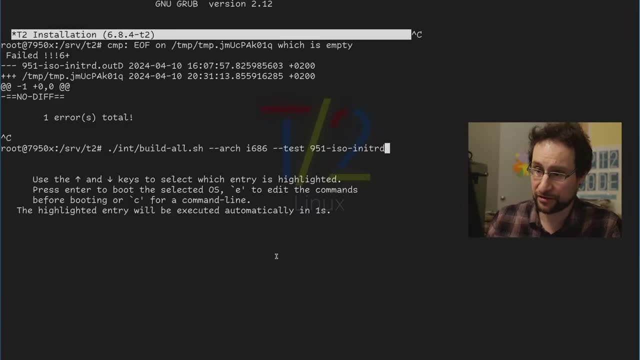 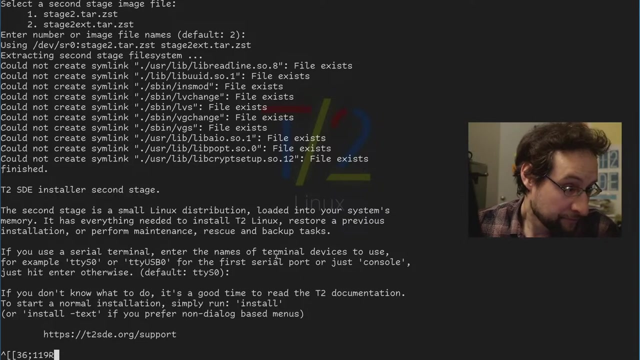 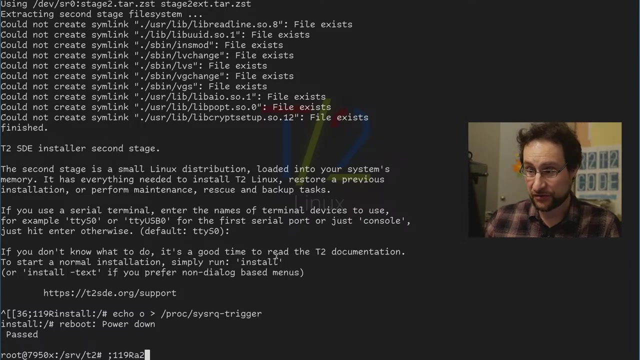 like to limit this a little bit of not other random stuff like 68 K, So 386 or x86, that probably should match right. Okay, Okay, that fixed that, So, and why can't I run there? So this test and also another test fixed amazing. 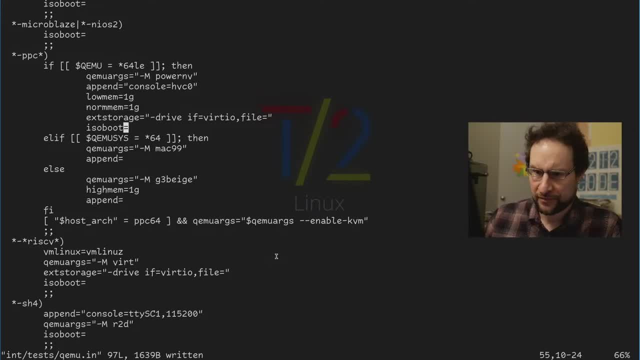 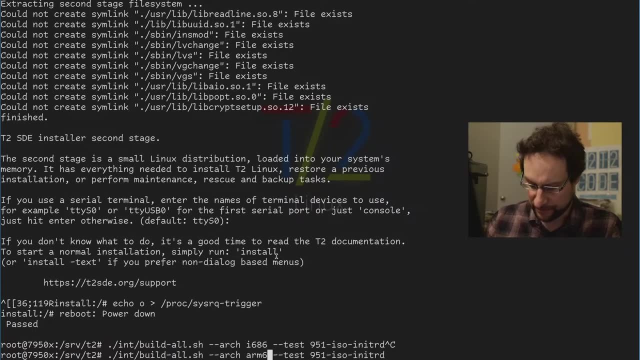 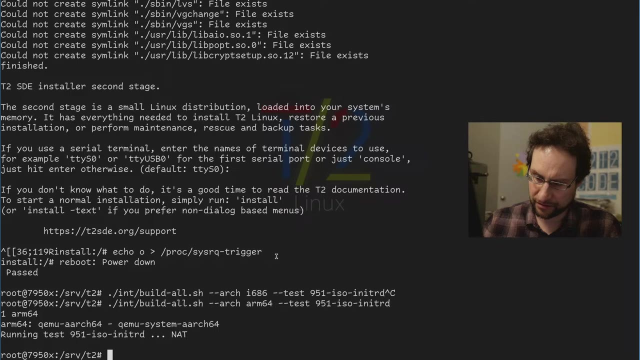 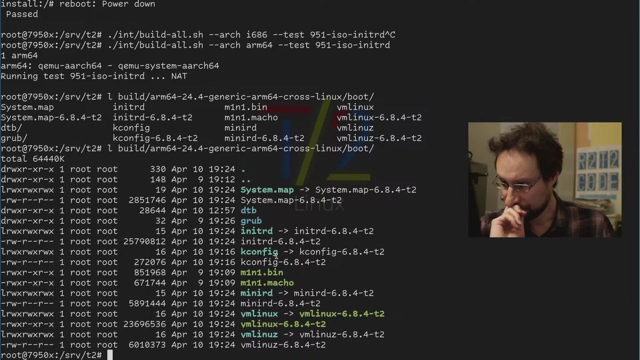 And then the one one more thing would be: arm does not yet work for this test, I guess. Arm 64, not yet a thing. why is that Not yet a thing? arm 64, this is not yet built. We have here slightly, or did. 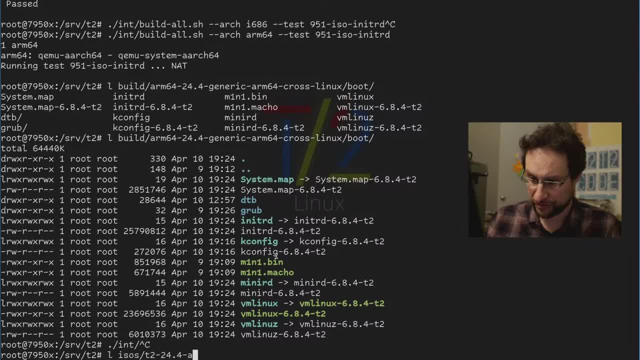 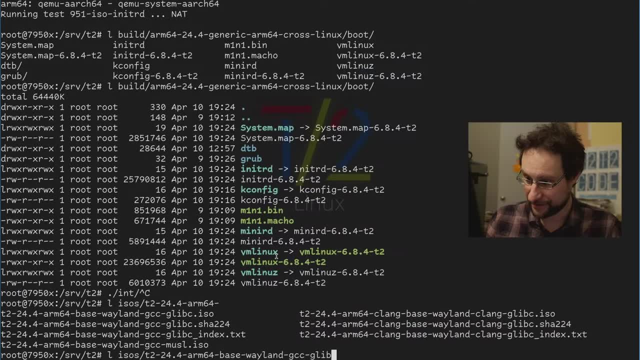 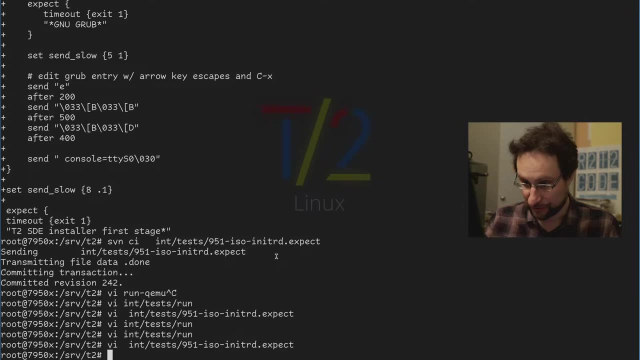 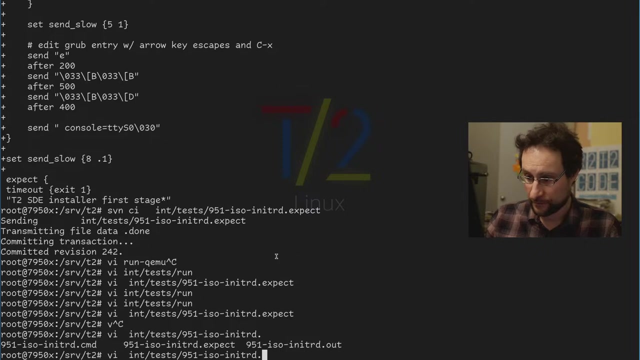 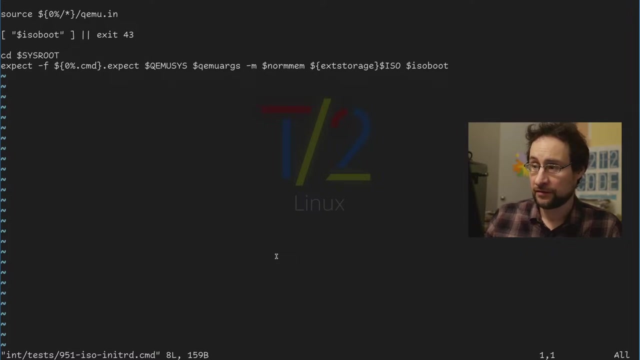 maybe don't have the ISO yet. ISO arm T2, arm 64, base. Yes, yes, we have many. no, that's there. What do we test there? That is a setup thing, for this is either: 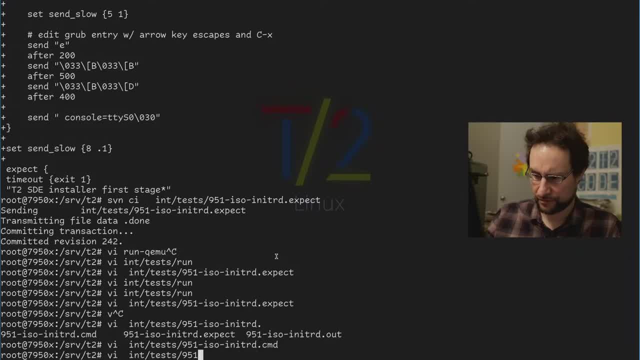 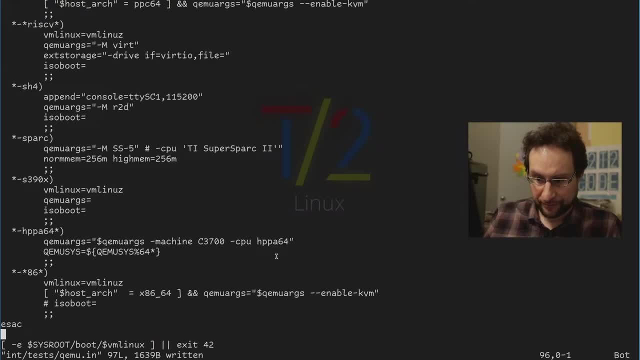 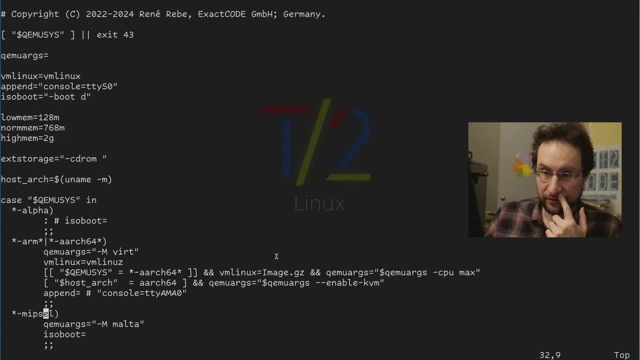 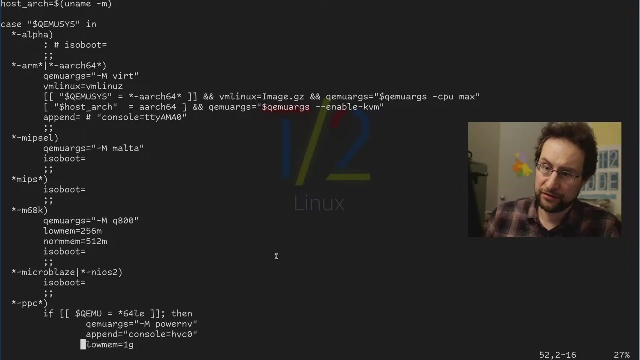 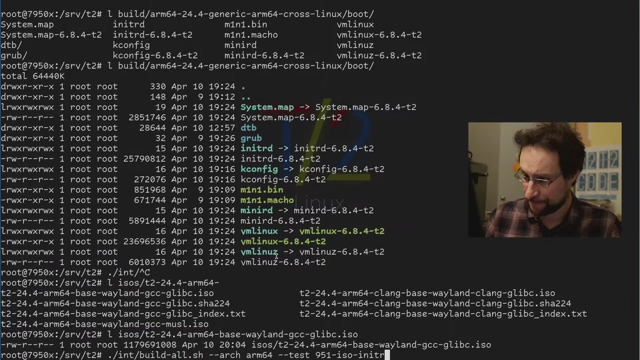 we do have that here, VN. do we match that for? do we even want to test the VN Linux here? So does this basically disable all the other tests? Do we have this? Yeah, I need. originally like re-next. 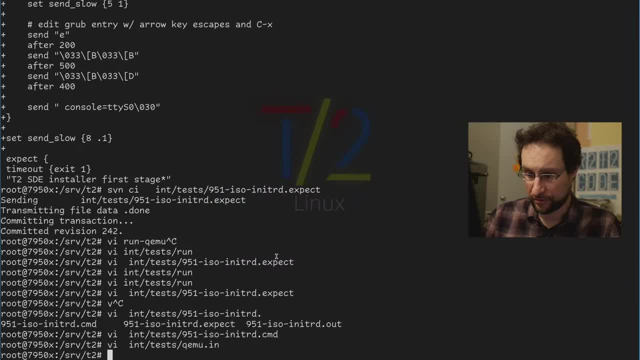 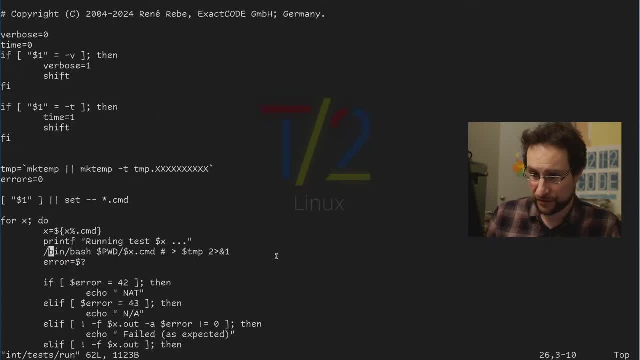 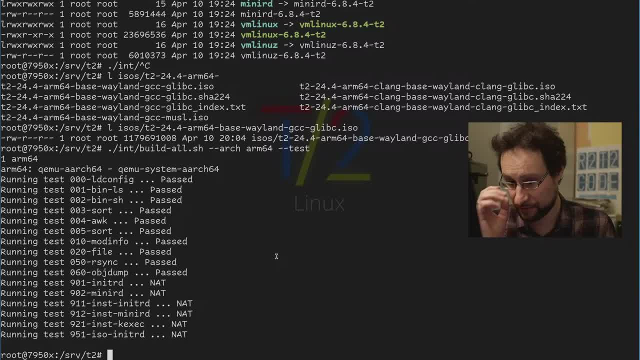 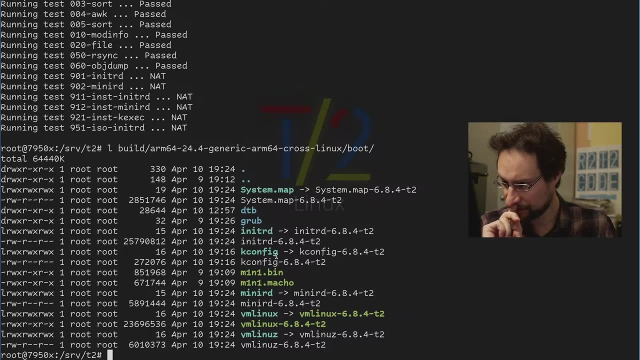 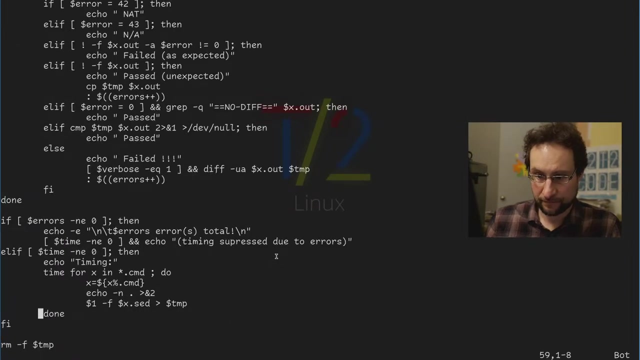 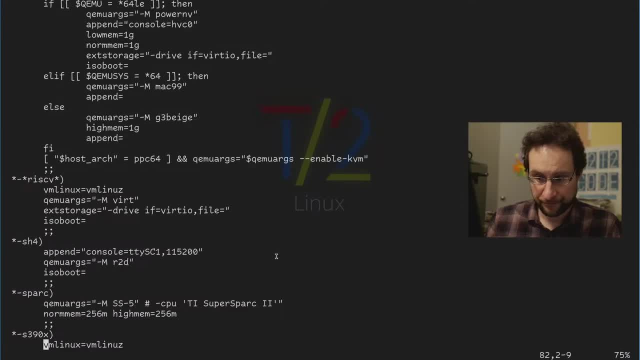 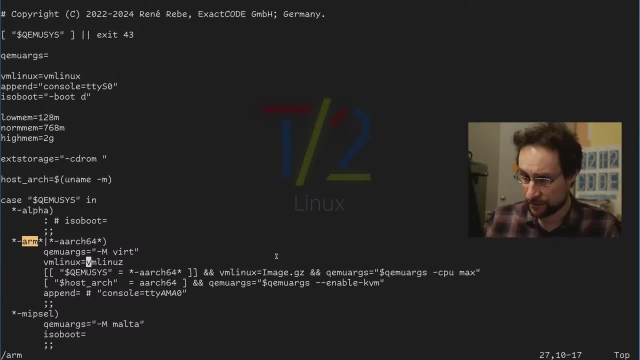 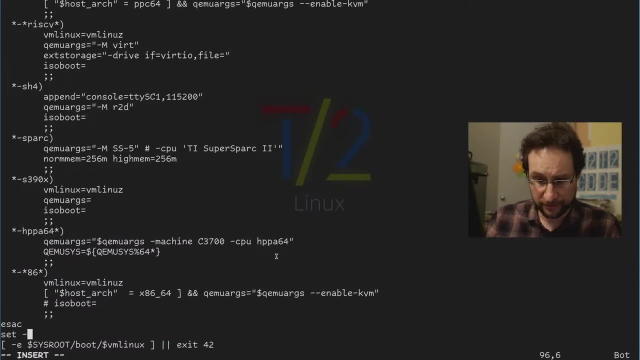 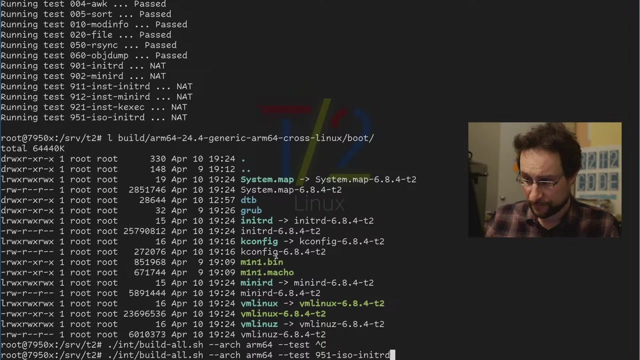 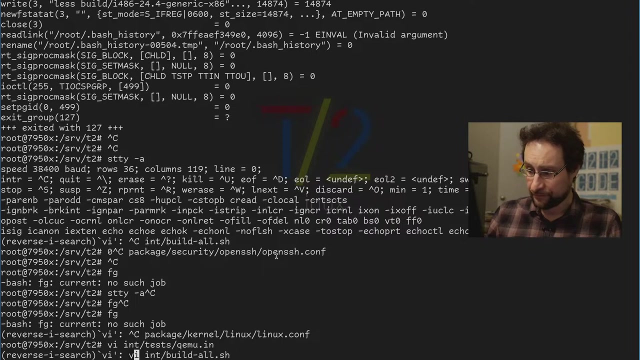 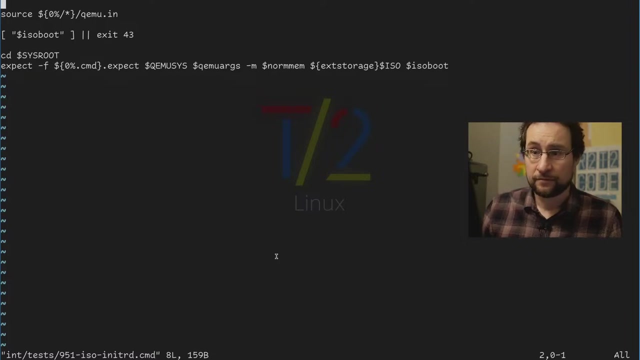 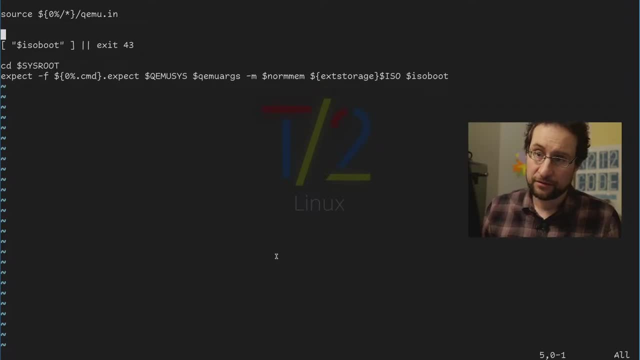 Or maybe don't tell me. I disabled that manually, but that would be 43.. Which exit codes did I use for Why do we NAT? not a thing. not a thing should mean. I mean, unless I had the wrong double. 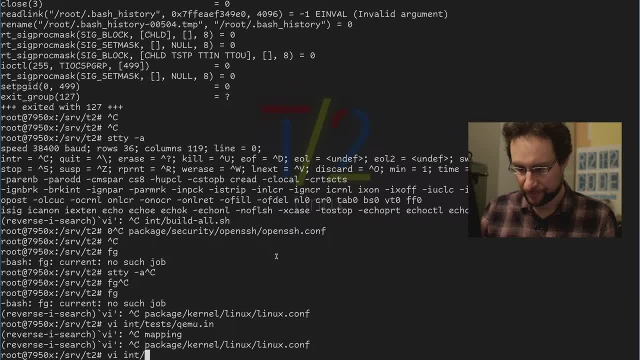 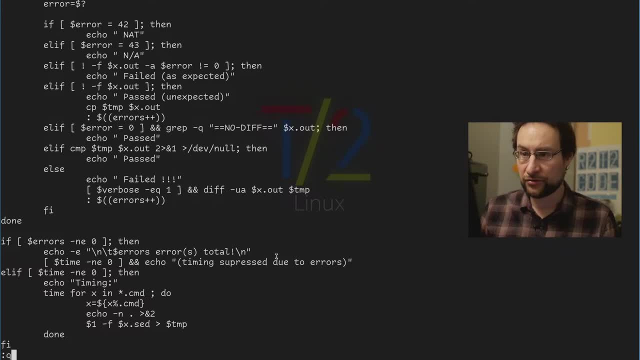 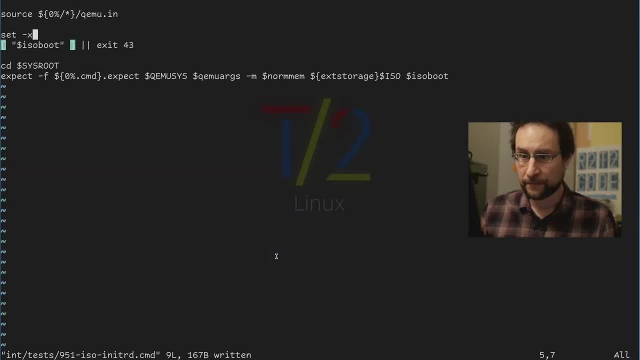 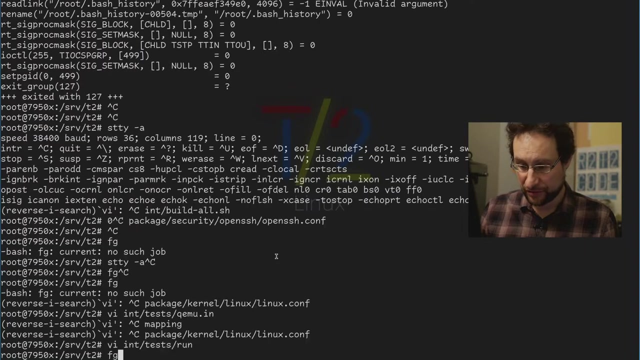 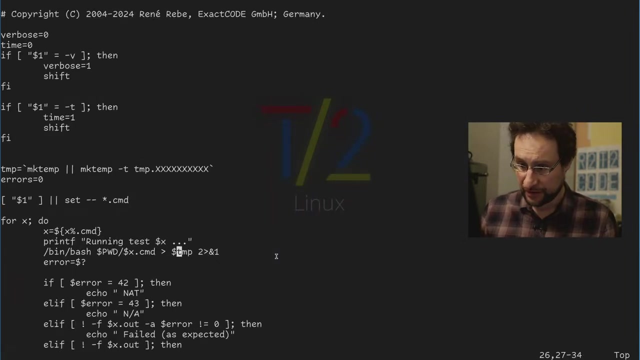 check set in the driver NAT. so 43 is not a thing, Because not 42 is not yet there. It's not set, though I guess we don't see the output there because it is probably hidden here. we piped this. 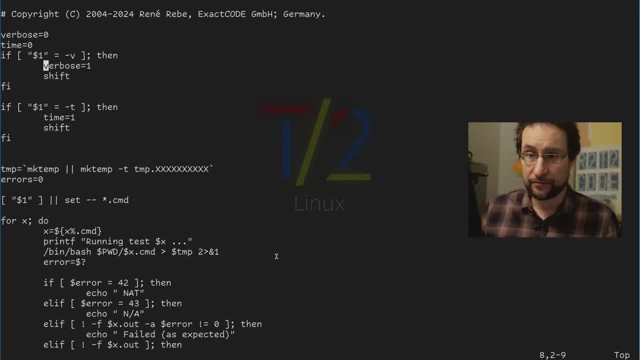 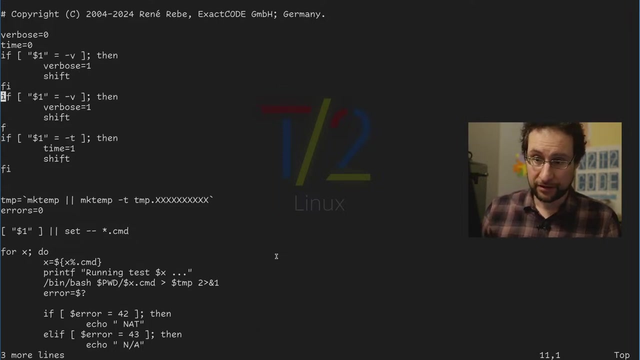 We could do this here, by the way. So we're both um like shift 1, so, yeah, it's a little bit low quality-ish kind of oops. makes it better later. basically, if we are still here, and I mean I'd need to also. 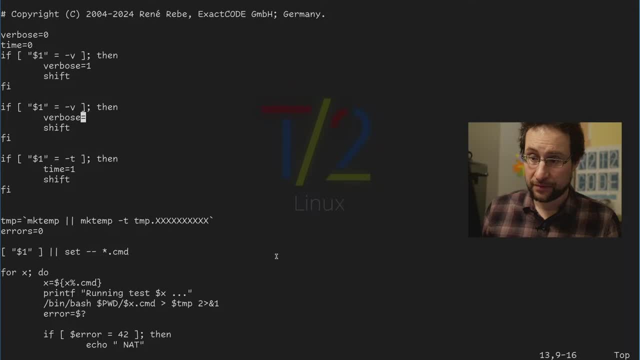 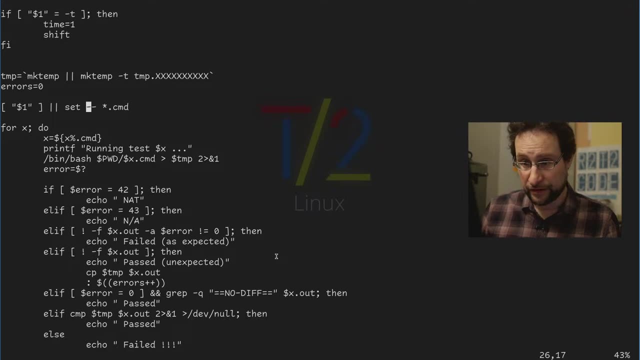 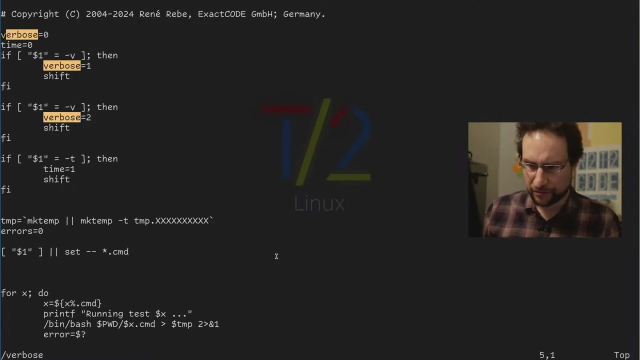 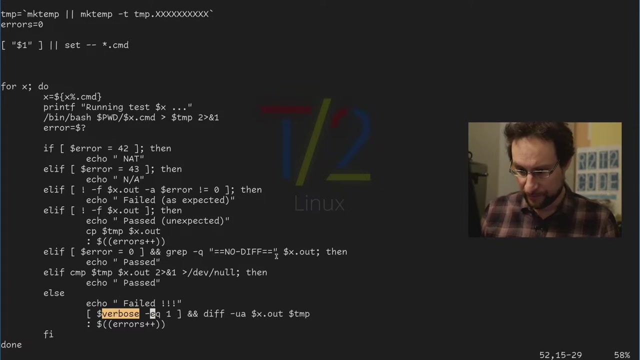 do that right then, but for today, I want to get ready here, Okay, Okay, Okay, Okay, Okay Okay, Then we could probably, or do we have no balls? do we only check zero Equal 1, um equal greater than 0.. 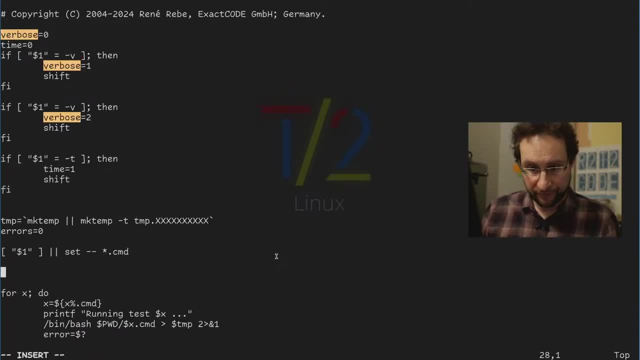 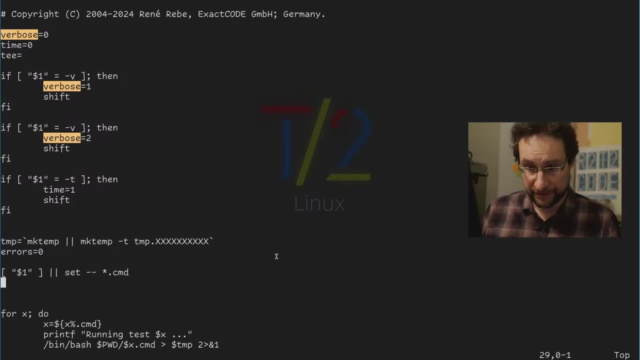 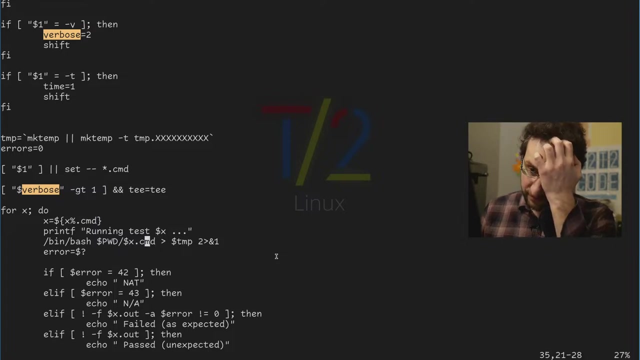 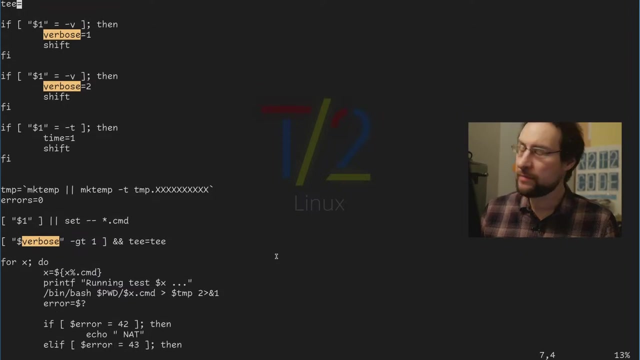 Okay, Okay, Okay Okay. And we could t0 and the both greater than 1, t equals t, right, I need to check how this even fits in there. to bash command, actually, we actually maybe better to this is this. 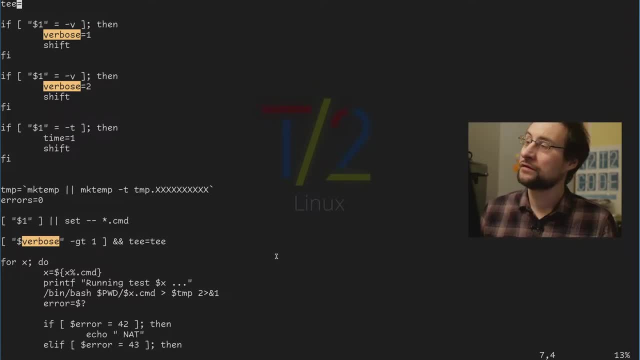 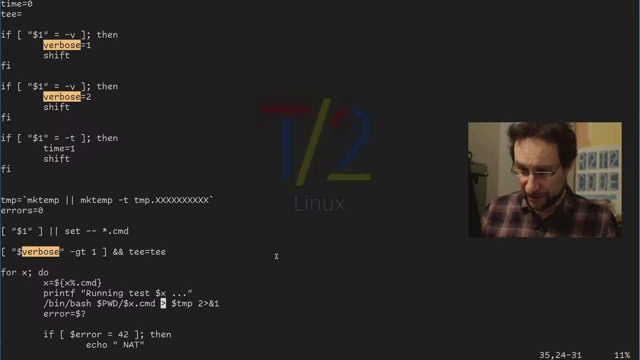 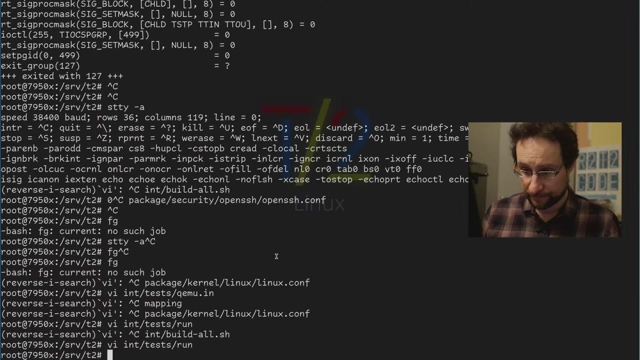 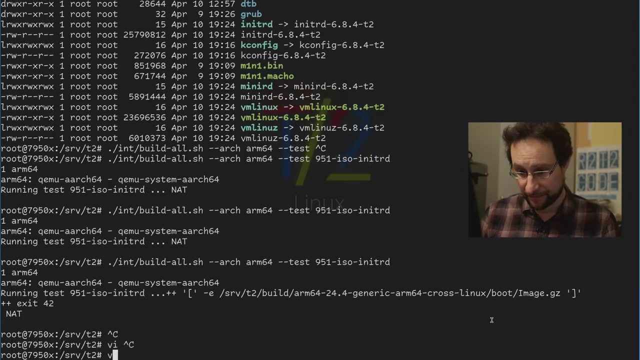 even standard in. basically, if we, that's a little bit more tricky. so, t or not to t, yeah, that is why I didn't. okay, finish this stuff later now. why is this? ah, I didn't. yeah, diagnostic is everything right. I read: 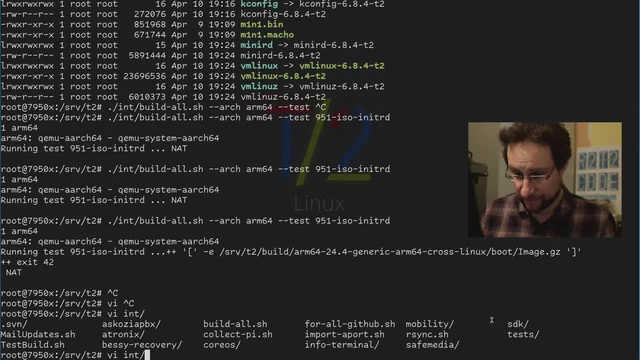 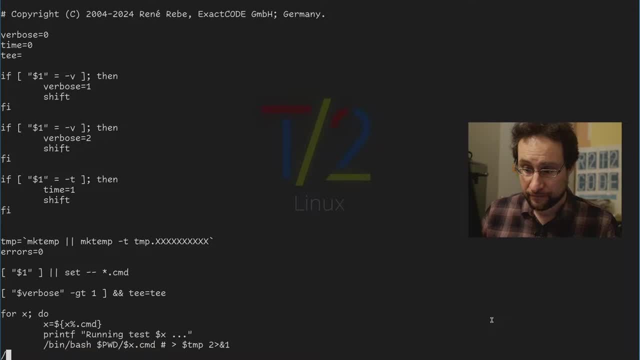 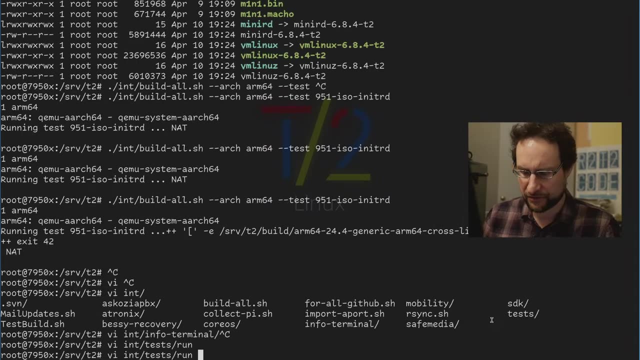 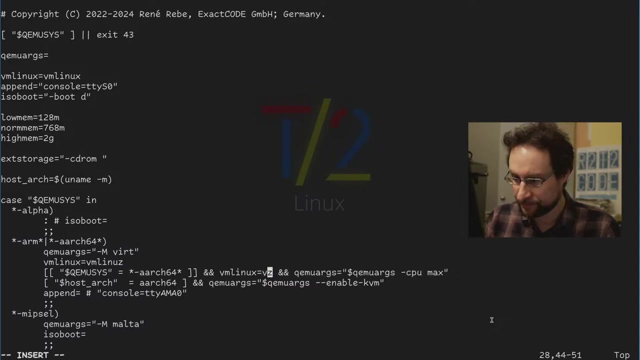 all of those images because the naming sucked. why is this not? where is this renamed? ah, this is also the wrong file. that is why so v um no, this. do we have set any more? maybe not? let's try that again. 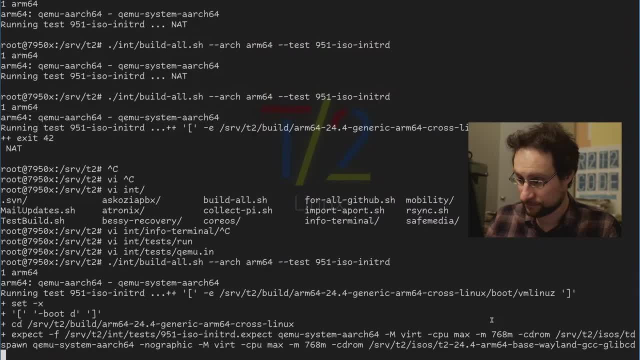 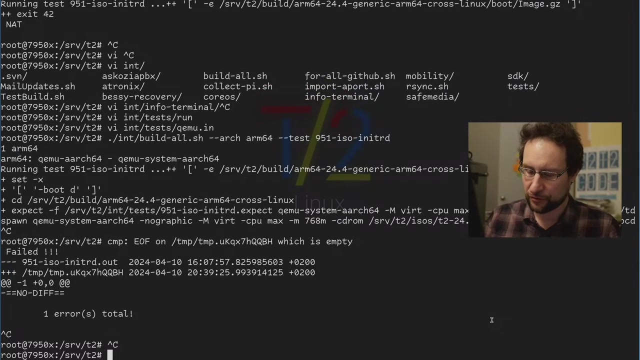 so now we run. so this might also not work, but it tries to um, so this is also what I wanted to do. so probably what do we have? iso? iso put um. this might be I don't know what. maybe it doesn't have firmware, or or non-matching firmware. 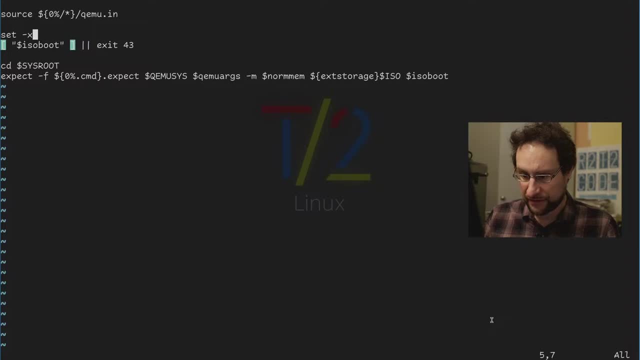 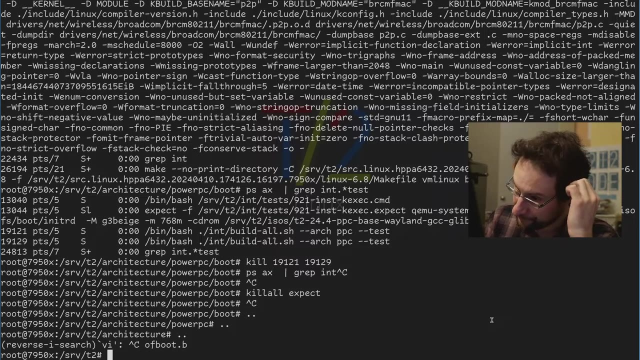 and that is also what I actually wanted to wire up. so for the moment we will. where do we run this um? for the moment, it needs the files need to be there. eventually we need um, so basically. 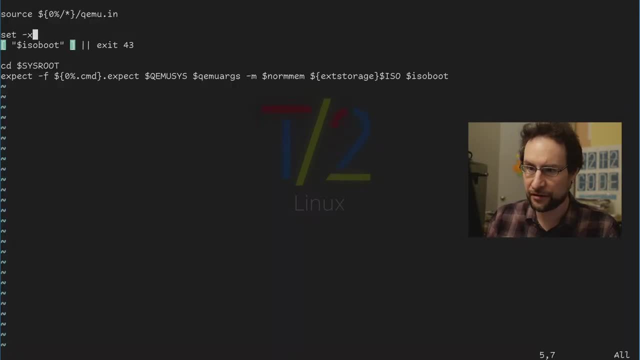 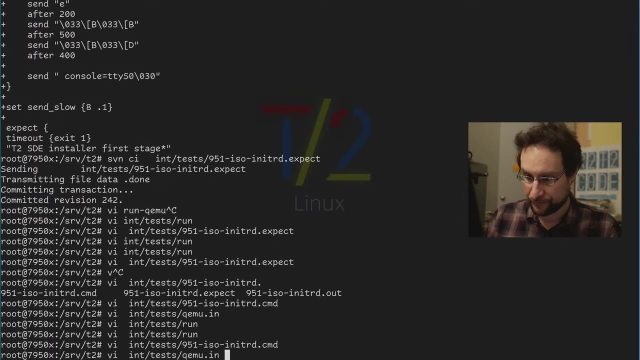 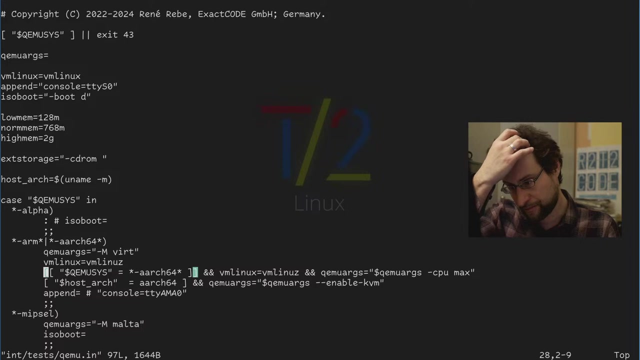 we need arch afirmware here. so um there, aarch, so aarch is here. actually, do we? we, do we need this? not for arm as well? I think, for arm we should also. 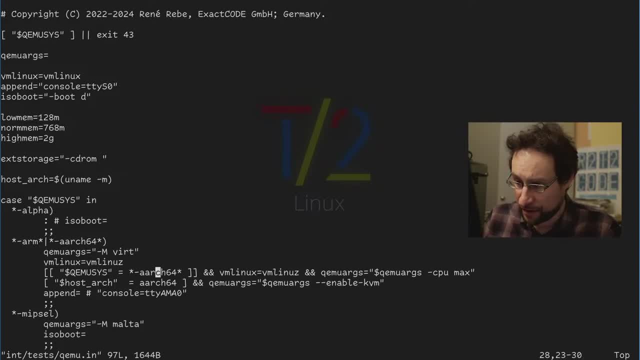 ah, we have that here um vm. okay, we can actually remove that because it is superfluous. now, as I renamed this nonsense, historic nonsense. and uniflats is also bootable thing as vm, linux compressed and whatnot. 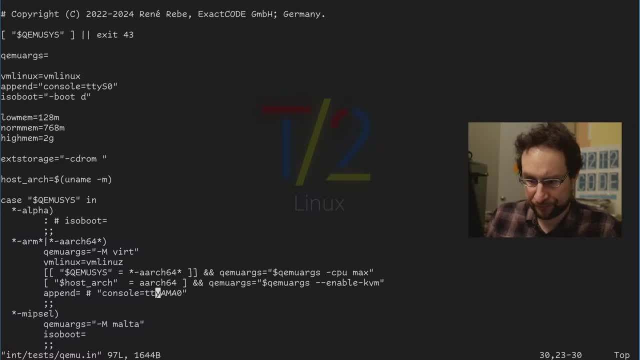 to finally have that done, and so this works automatically. um, okay, we don't. ah, our documents is documents, is not so what did I want to do? I wanted to do so. aarch, host, arch, aarch. 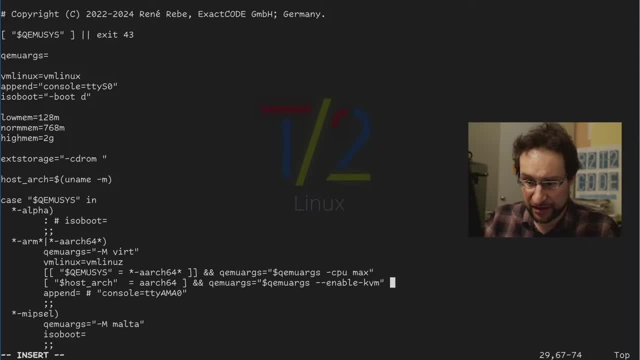 q, emu, arch, emu, args, that. and isoboot equals bios, in which I need to check which directory we run this in now. so so that, like, basically this is getting too long right. 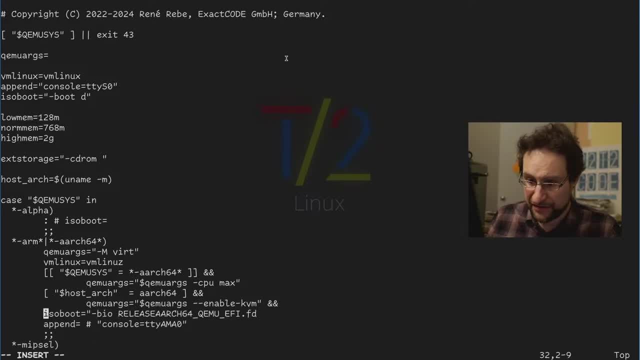 and so we don't wouldn't need end there but to have this line break there. so bios release this stuff and the rest of isoboot. we might need this if ifybios thing for more. 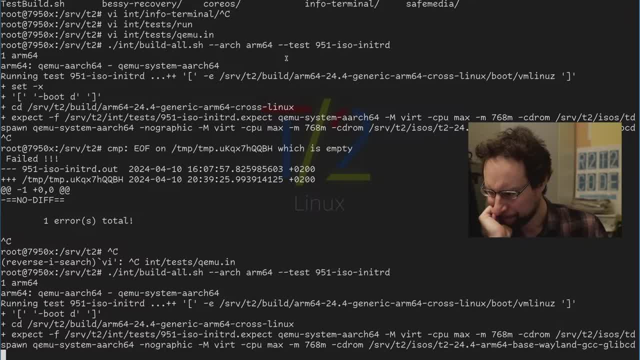 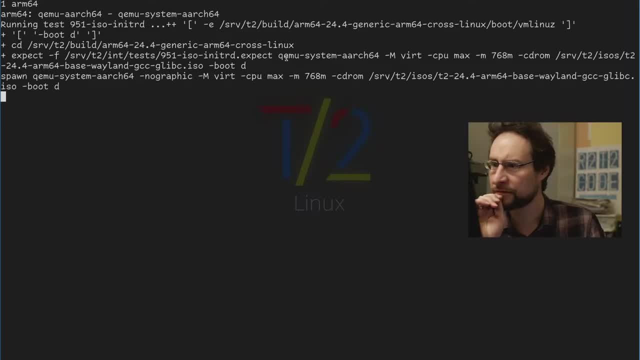 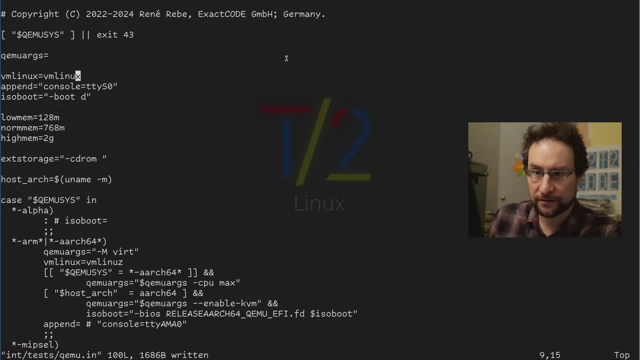 but for now does this work? maybe not, unless it is some line-wrapped stuff. what have I done here? arm 64, host arch, isoboot, arm or stuff, host arch. oh wait, this is enabled. this is in the wrong one. 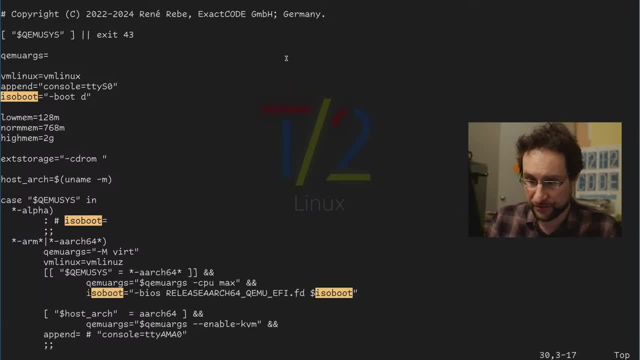 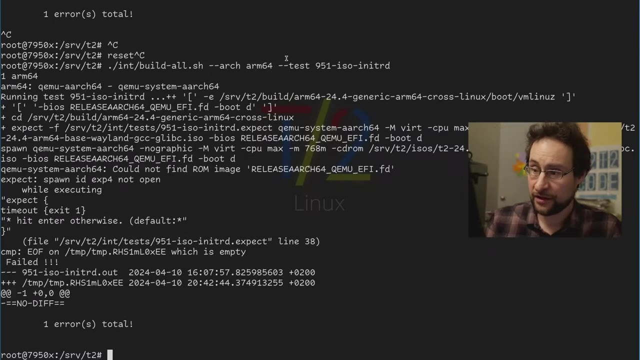 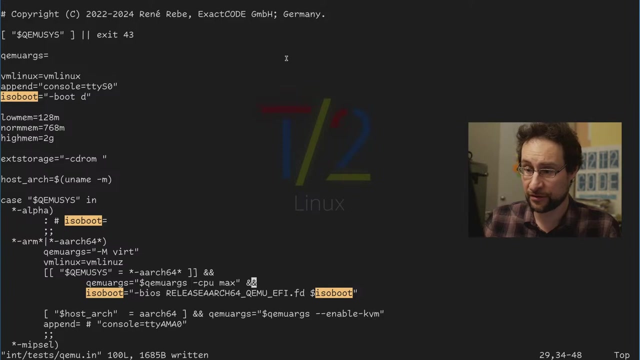 this is only if you run this on on arm. host did nobody realize that, so that doesn't work. in which directory do we see? or we run this in the build directory, because that is what I wasn't the most sure about. 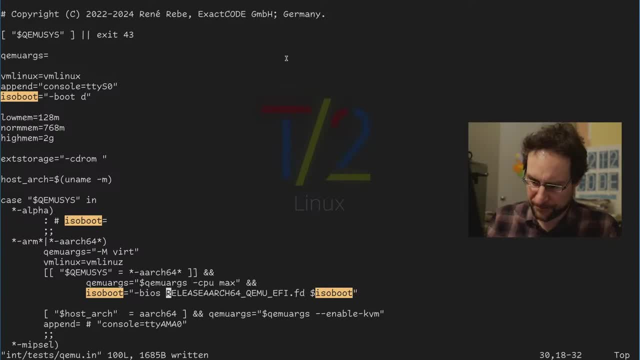 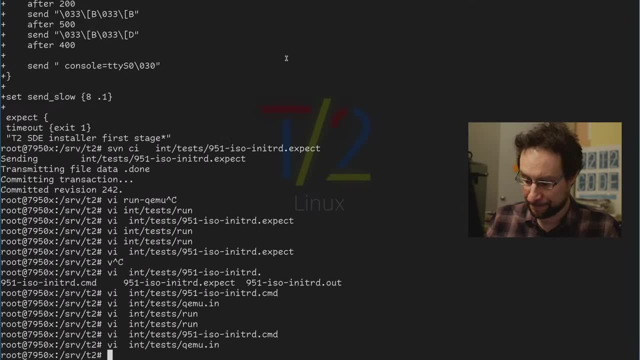 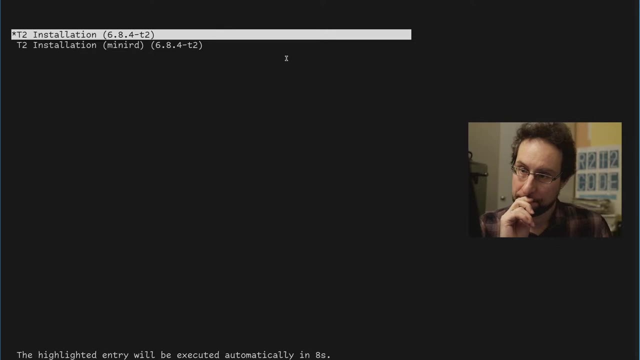 so then, for now, so later, we would like to do some unified place, what not? but for now, for now, there, for my testing. I'm going to go to my library in. let's see I'm going to go to. 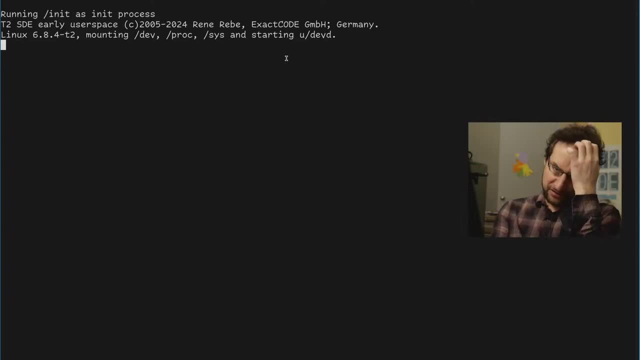 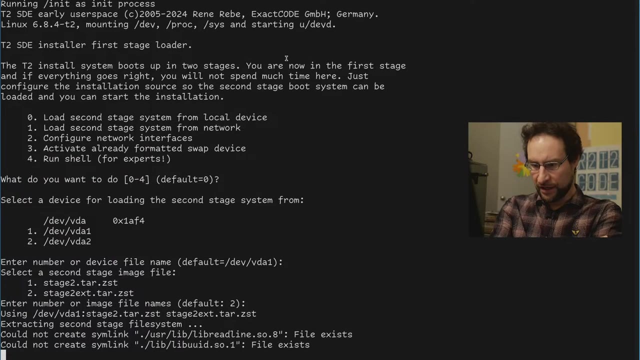 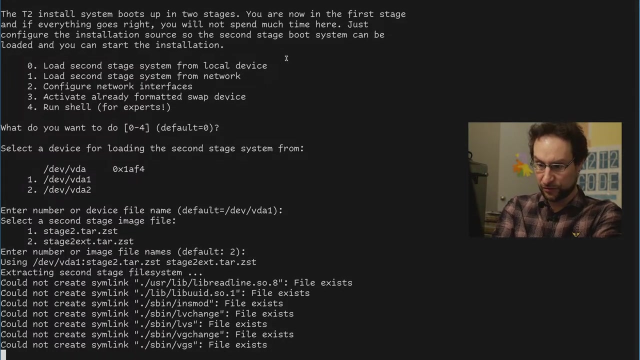 let's go to my library in and just like that this will do, and then it works. so let's see, and so I have currently 30 seconds or so, I believe, for the whole, which is also on my to-do, like next, we need fine-grained. 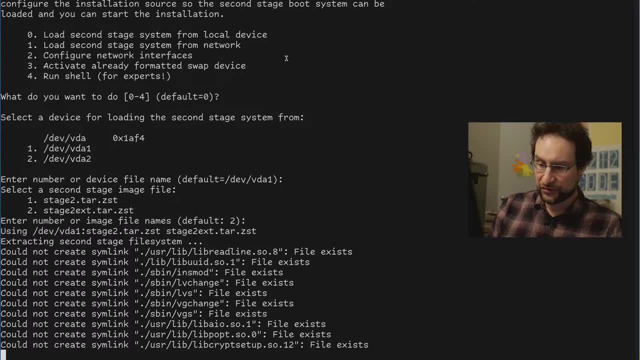 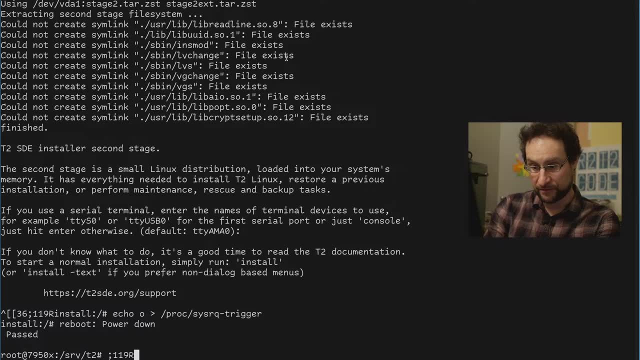 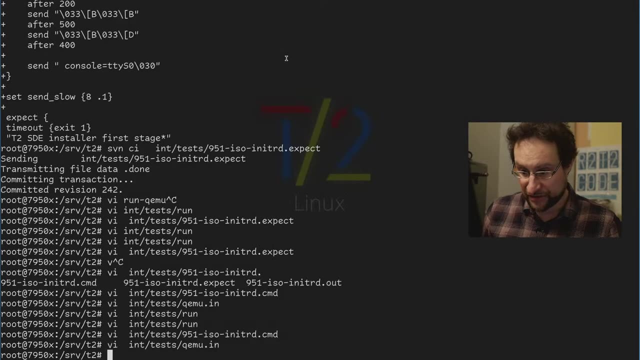 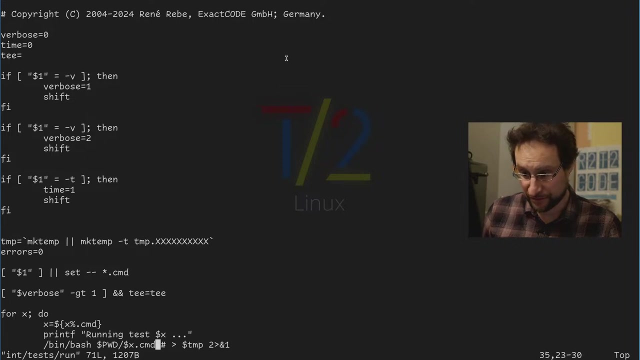 fine-grained timeout between all of those We probably managed for some reason. I believe I have 30 seconds timeout, but amazing, cool. so Theoretically we could actually test like that. Let's change this test driver back of putting it into the file where it belongs, and 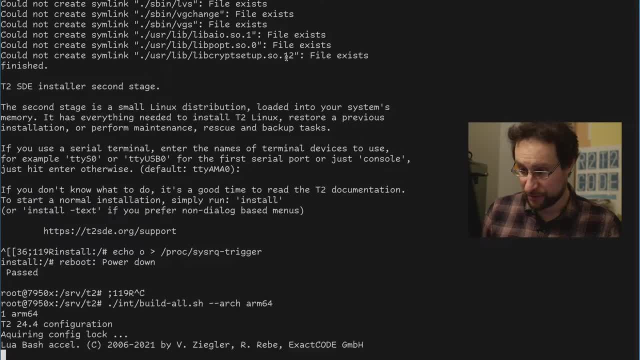 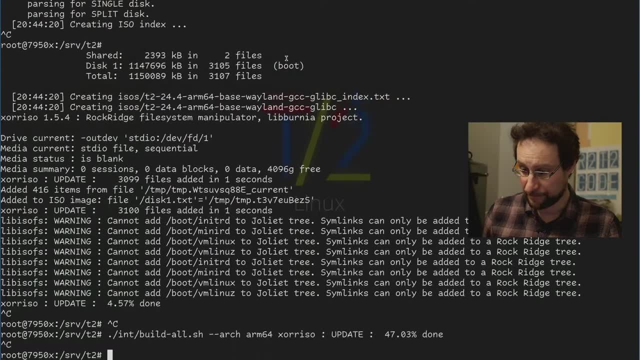 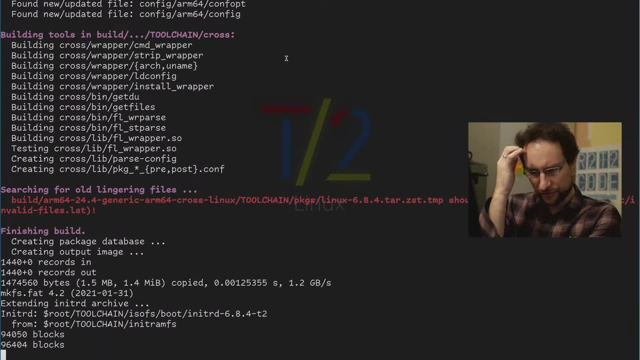 Then let's. I believe this should be all. Oh wait, I did this wrong. Okay, now we. Okay, now it's. It was still generating, I believe. Yeah, because I ctrl-c. Yeah, okay, We better to have the whole iso, otherwise I missed the iso. 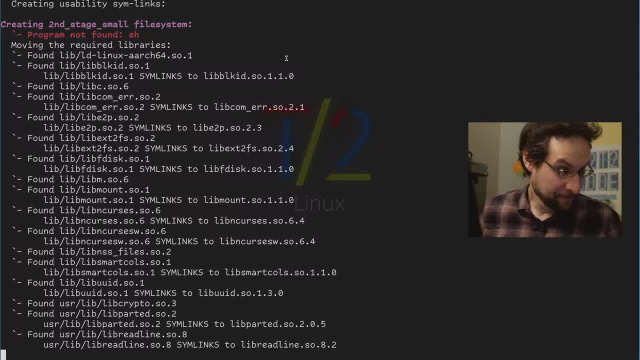 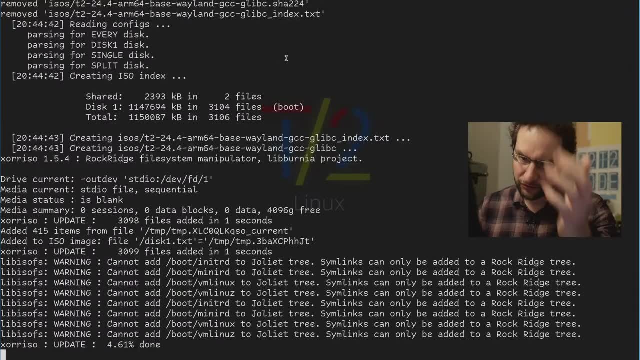 Only life on this channel. trigger happy on ctrl-c. Yeah, that's, that's how you do it, right, that or that or similar and leave in the comments below: What do you use for your testing. Do you unit test? Do you do you think you do unit test? Do you unit test enough? 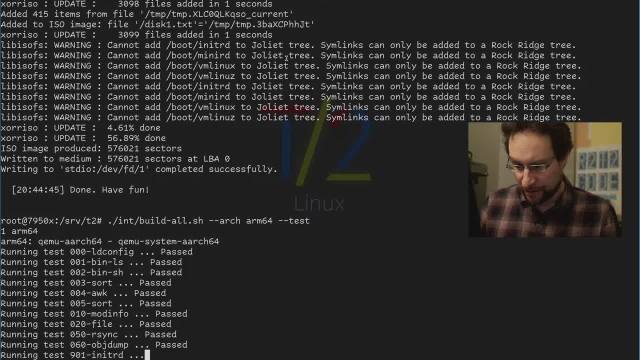 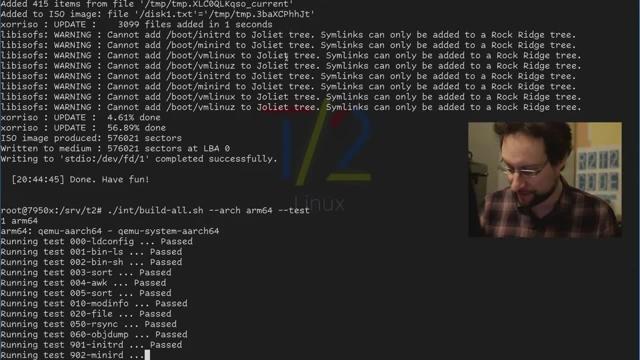 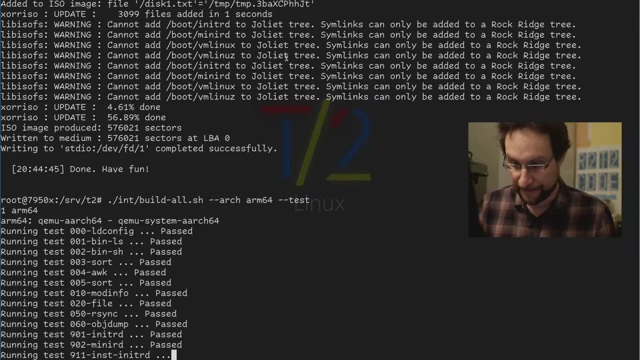 That is what I wanted before I messed up the iso. Okay, but the other test probably also pass, Except kxl. kxl is broken on most architectures except x86 for reasons Increase upstream right used to use to use to work for power, pc and arm, but no. 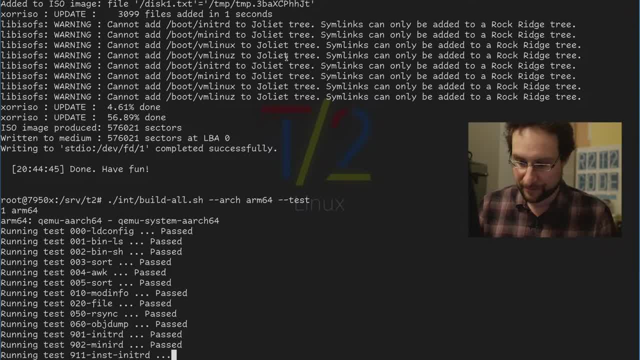 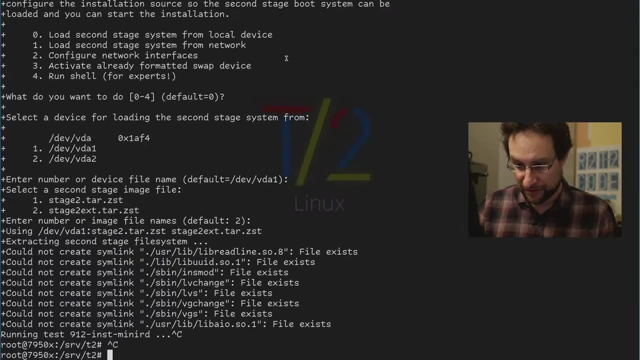 and of course, like yes, theoretically native high-end arm silicon kvm- right, It is what it is, so In it Rd. So yeah, that takes. I mean, the other will take nearly 30 seconds. So sorry, one like kill all the stuff always, so it's. 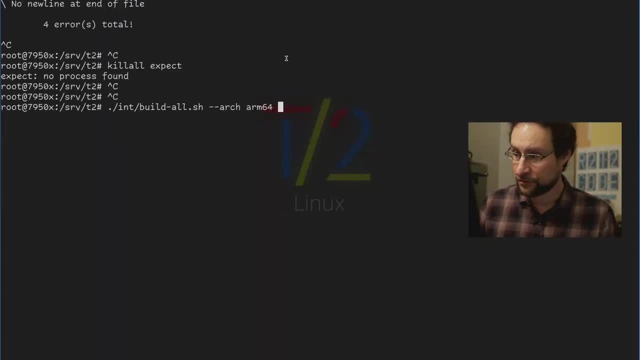 Do we have killed all here? So I would be more interested to run this new test for all architectures. that would be that do that for all tests, as 951 is in it already. but that's basically for today. One other achievement check marked. another achievement unlocked. 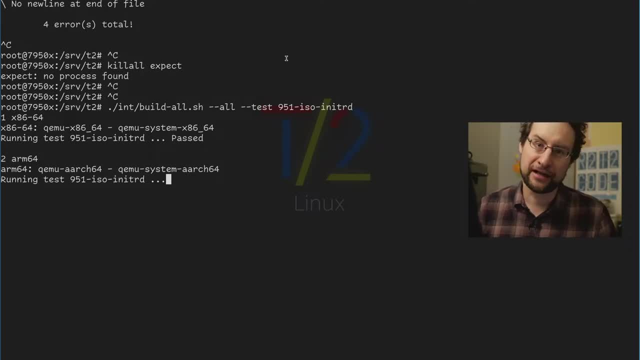 I hope you enjoyed to learn something that is like, yeah, all the effort, like not only doing all the stuff for 25 years, fixing all the stuff, but at the end of the day, sure, decades ago we wrote we burned ISO data on optical spinning meteor and like that certainly. 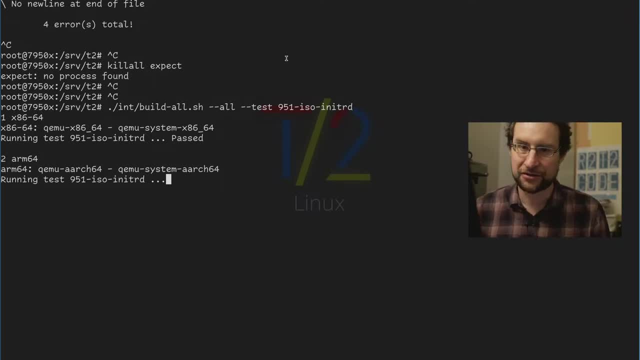 didn't scale very well, except unless you have 100,000 or 10,000 of developers and users that then break their hardware. If you have any ideas for improvements, leave in the comments below like: do you also tickle, tick, tcl, tk, expect or use something even more amazing? 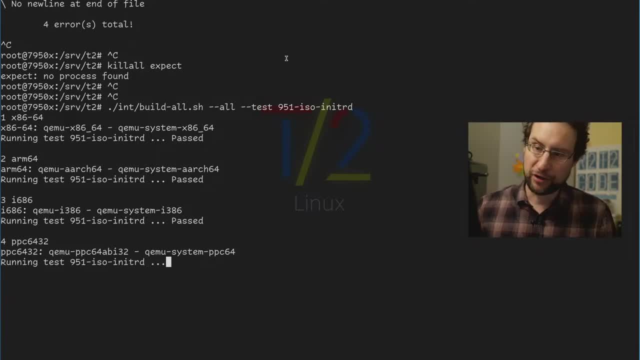 Yeah, we could. so for improvements, this stuff could run parallel right, which it would, for it's a whole test drive or build. all driver has already parallel run. Visualization, I mean very theoretically. if you wanted to do ASCII art, you could visualize a table, and just you would need. 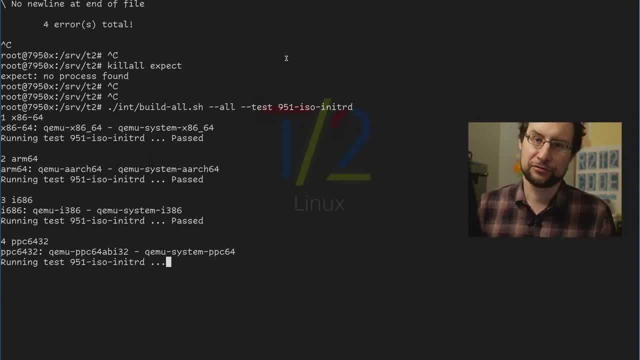 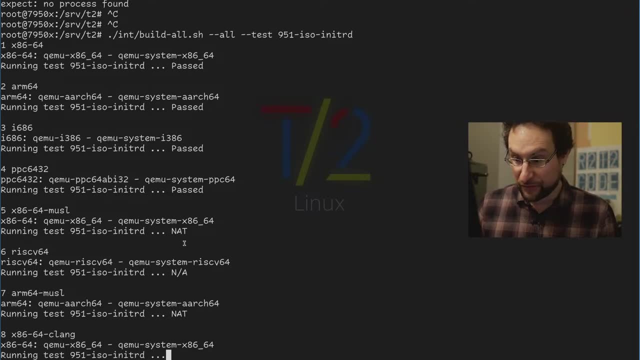 like to do all the quirkiness of capturing all the output, making sure it doesn't print random stuff there between and so on and so forth. So, yeah, risk 5. so we would need, so this might not yet be. yeah, some muscle or so built I still have. 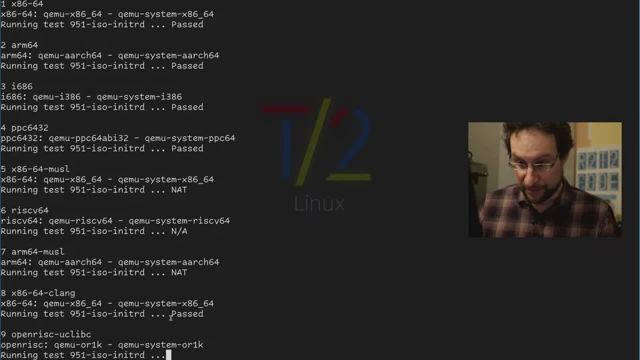 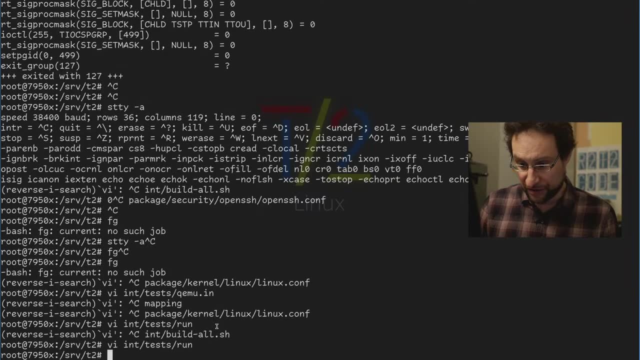 to fix some stuff. Um, hey, is this even passed? Was it relatively fastish? Failed fastish? Probably this doesn't boot. um, so that is also why I do this right. so we still have some annotation to do so, Or a 1k or something. 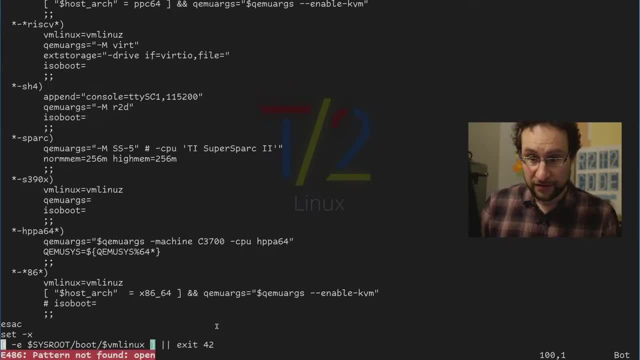 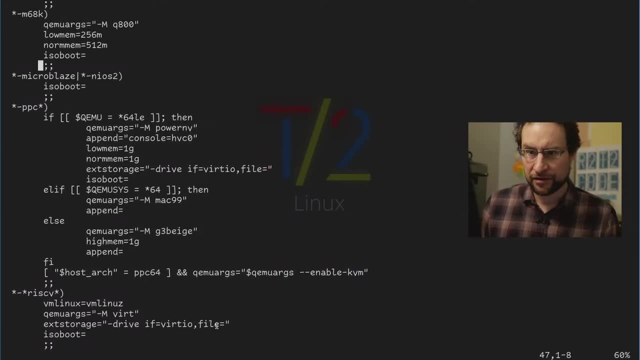 Okay, Okay, Okay. or open risk, don't have that. even do we have somewhere disable isoboot? catch, all are here, so that is open risk not. or open what was a short form for that, or one okay, probably like that. no isoboot for that, I guess, mostly 486.. 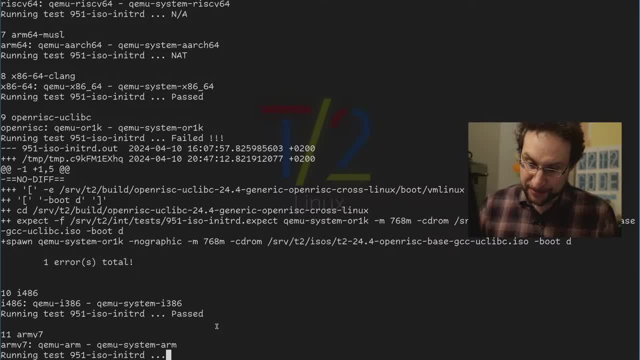 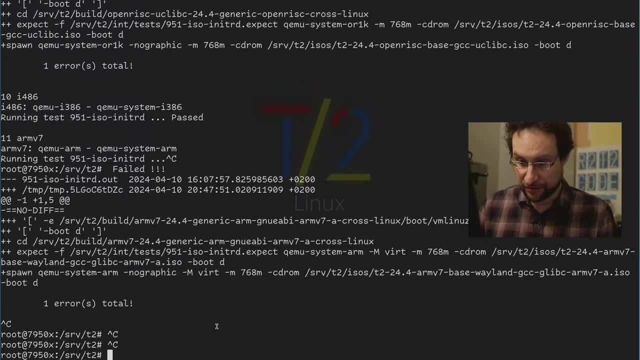 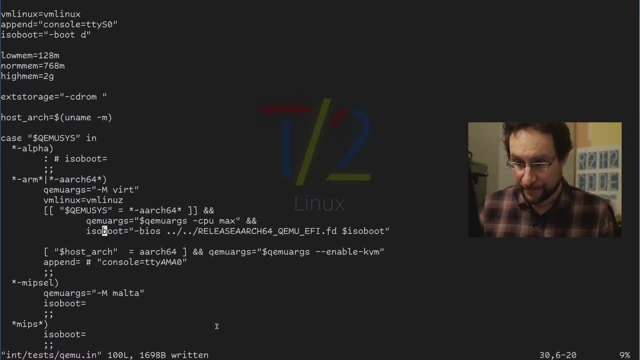 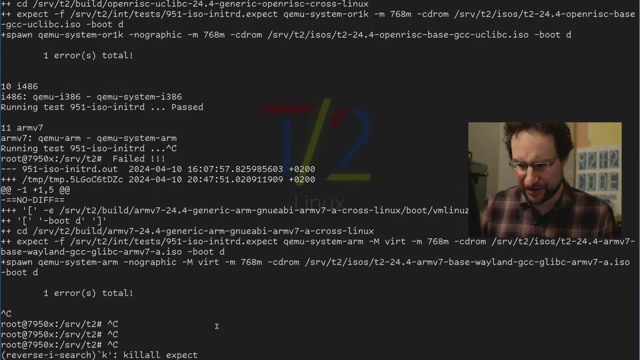 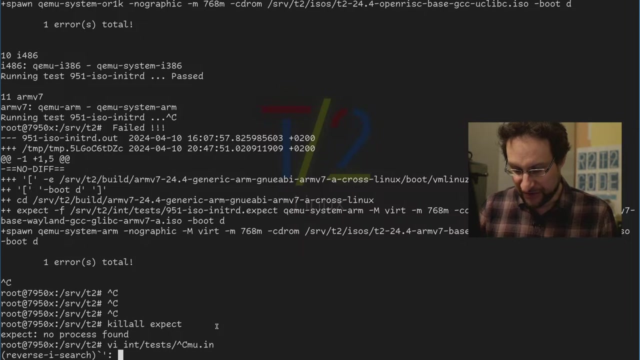 486.. Also passed: okay, the arms, things will not pass um. I can basically control, see that. uh, so that is that. otherwise, we like, what do we have here um something? um, I, I pre-tested that for that, that's basically. we don't have an cd bootable bios there. 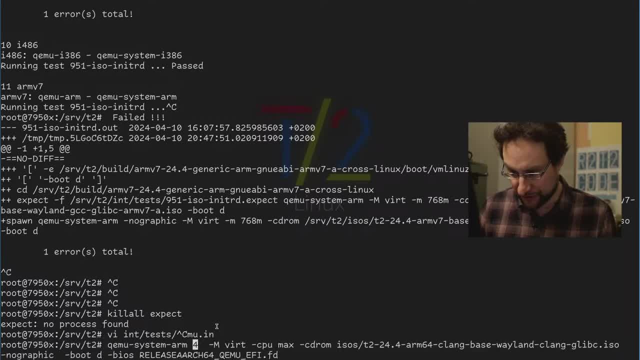 hey, arch. so I tried to test this. it didn't work. so we have here some release arm if you buy a thing. it didn't work for me, I believe, but we can double check that. so this is arm: mvert cpu max max for arm. I do not have a better way to do this. and you can double check this 1-th person and you can double check this 1-th person and you can double check this 1-and 2-th person. 0, I mean, I guess, yes, field 5 comes there. 0, I mean, I guess, yes, field 5 comes there. 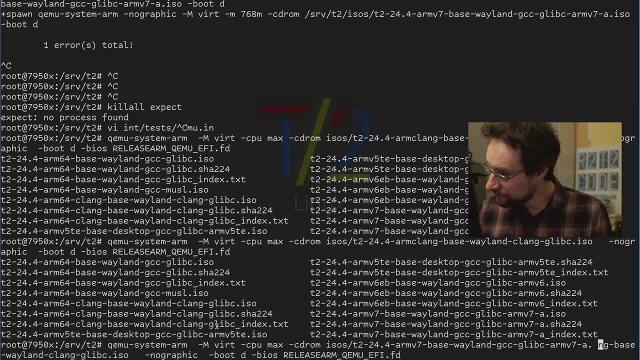 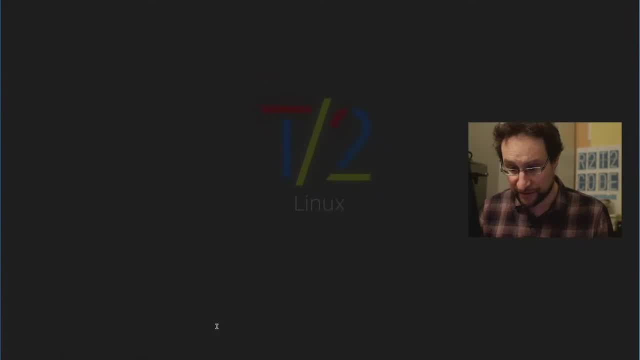 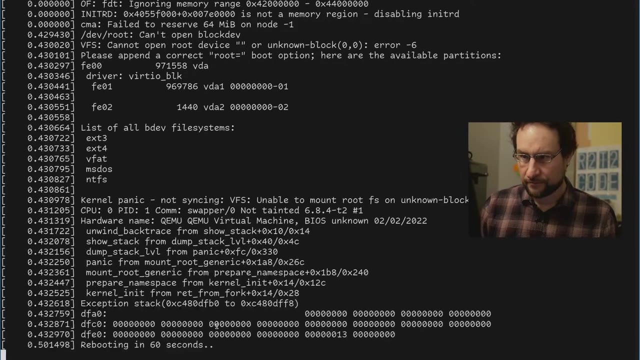 0. I mean I guess yes, field 5 comes there, so lose. so so this one in my bag, let's see we should drink if we don't use that anymore. drink, dan y Sri, drink drink. they wrote me on Instagram. they wrote me on Instagram was just okay. this doesn't have an in it already, for reasons. why would that not? 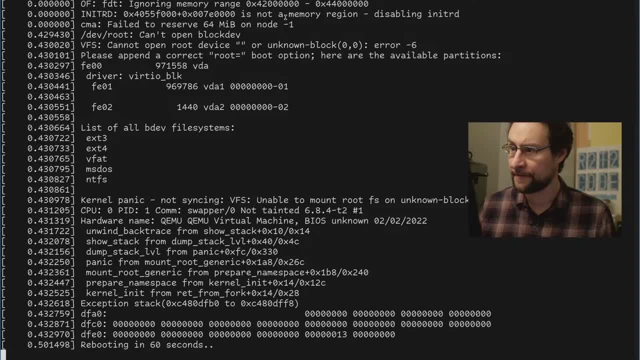 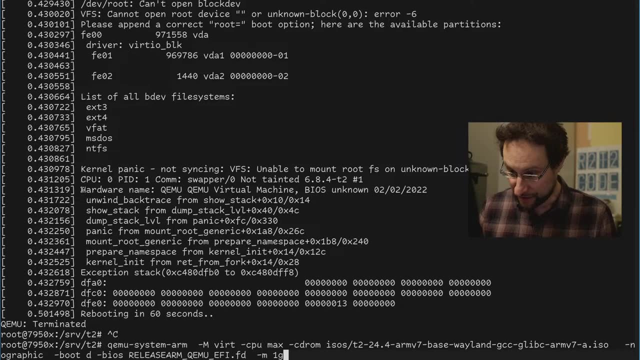 have an in it already. I mean it boots mostly. it's not the memory region disabling so fat, so some. how it's out of memory. ish did or maybe didn't. okay, maybe I just didn't give it enough memory. let's like this. okay, let's copy. 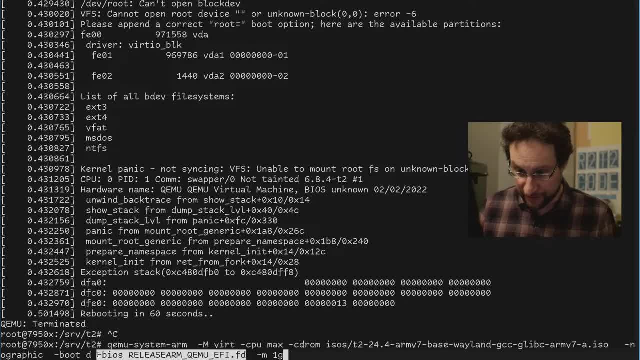 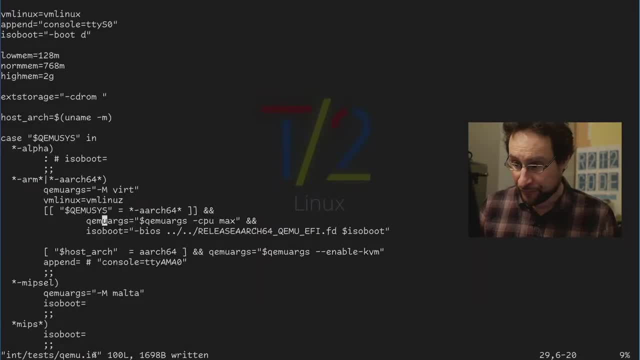 this. that's a nice surprise. let's see if that works and we can also. so if I better, I mean I could at the zero getting a little bit convoluted and error-prone, right. so we move this equals arm. I should should be nothing, right then? I support equals, that one boot, I mean. 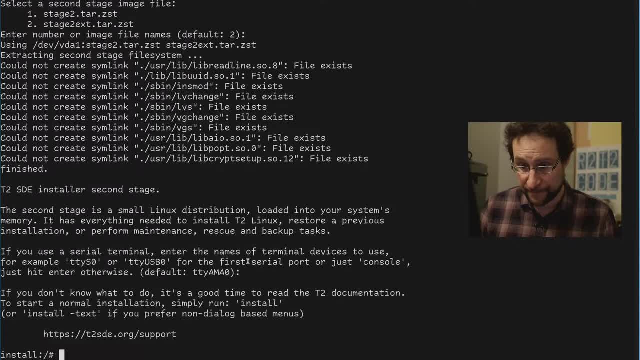 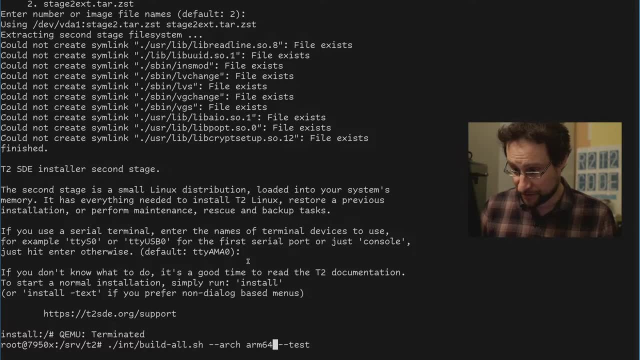 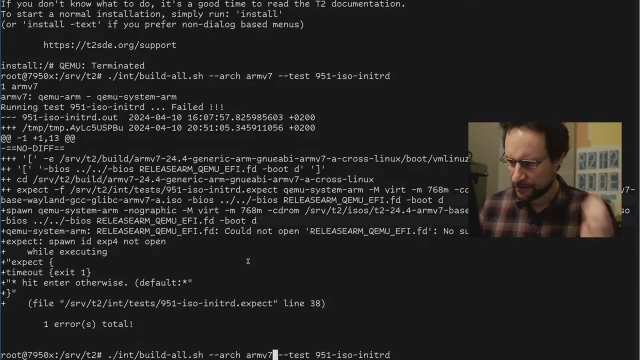 here it's could be more generic, so amazing. then we could actually test that, I, I. I have one more test: version 7, right, all right, we want this test prefix for version 7, plus variance on version 7. what's going on here? couldn't open dot. 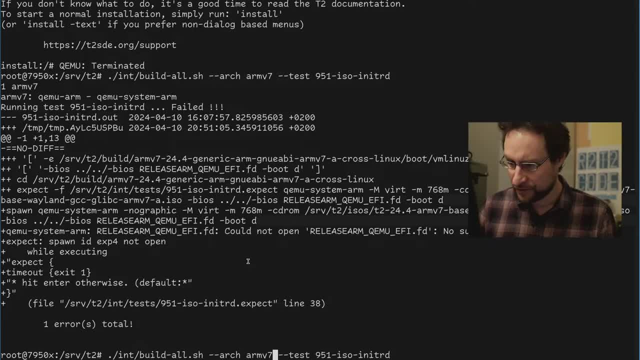 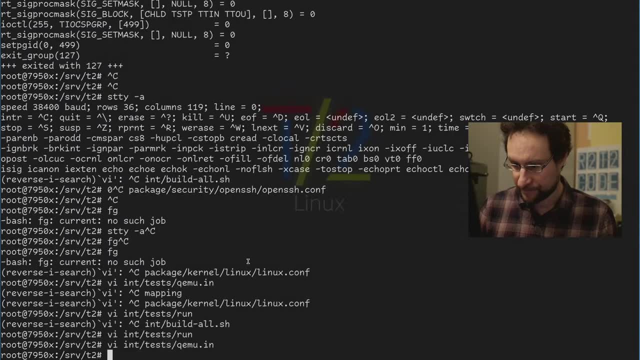 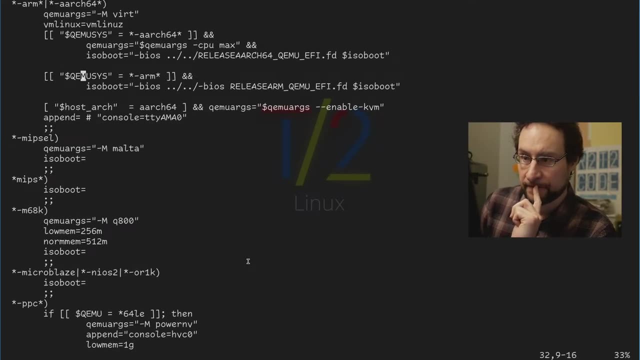 dot arm and stuff. what did I do? BIOS are some of these types of problems I've seen, so we need to find it. so I'm just gonna copy this test case. what did I? what did I? let's type here. it's on white, copy and paste. I just want to say: let's see. 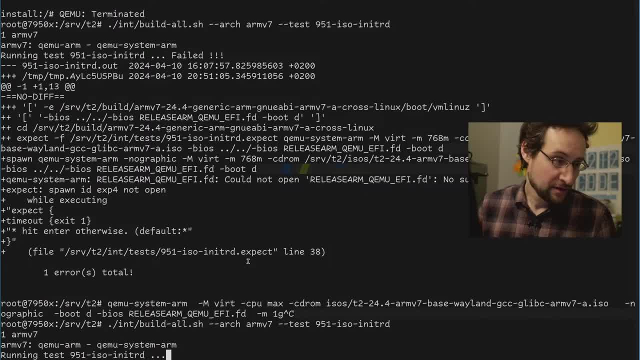 what's going on here? what did I? let's type here some white copy and paste fail. that's better, maybe that's. I've run 32-bit ARM EFI. it's like hey, even works in QMU, which means that's certainly some. 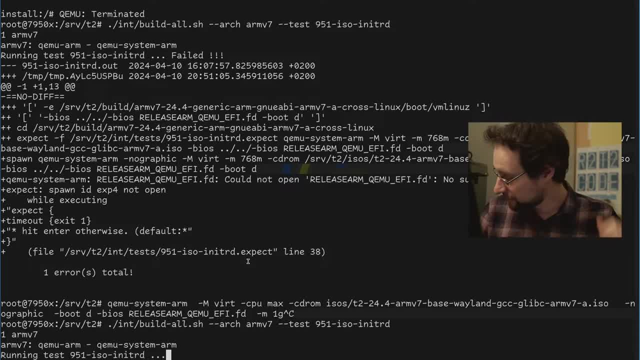 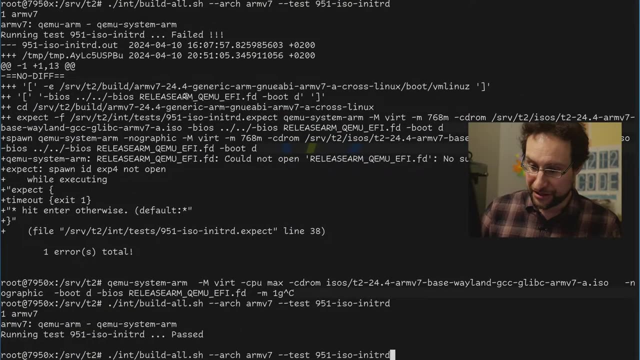 nice thing to also keep the ARM stuff a little bit more tested. So yeah, that's basically it: Another day in my life spent on the effort of supporting all architectures and really, really actually working and test the Linux distribution. I hope you appreciate this and. 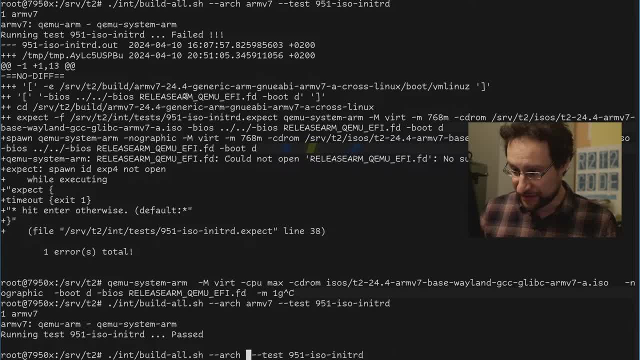 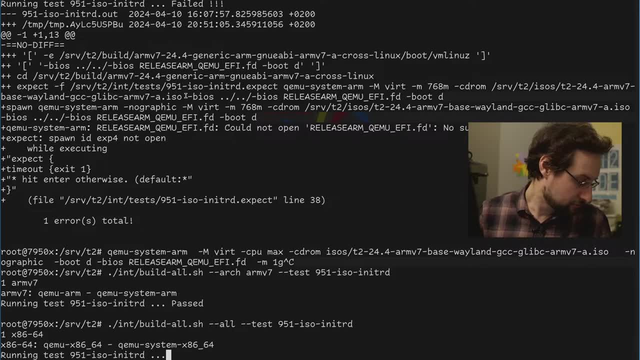 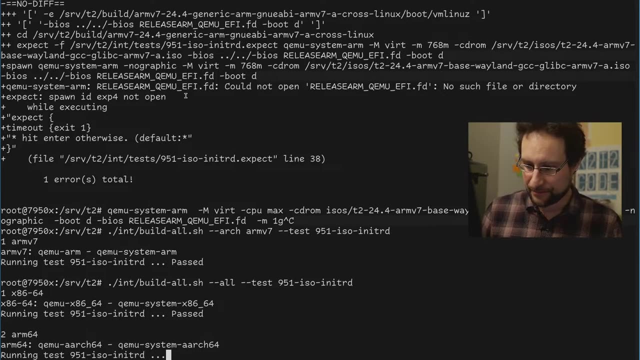 have this, even freaking, worked like most of the others. So, yeah, I could run this once more, see what else we fail or not. Certainly way, way more room for improvements. There's always like 666 lines of to do and bugs and to fix and features to implement- Probably another. 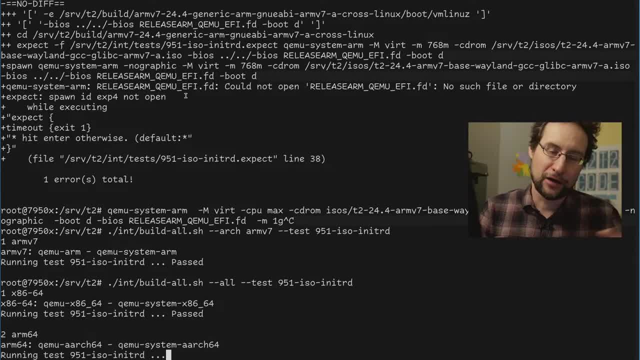 yeah, 45 minutes I mean, and that is with four hours doing stuff on Twitch and one hour in between working this, sending escapes in a humanly slowed down way for the slow QMU menu redrawing to work. Hope you enjoyed to learn something. Don't forget to. 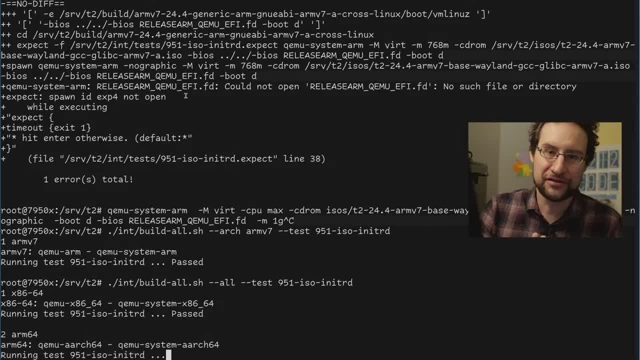 select subscribe, and I hope to see you soon, for actually what I will do now is arsing the ISOs to the interwebs for you to pre-test, And I hope you enjoy both the videos and to see you soon for the then differently interesting videos. 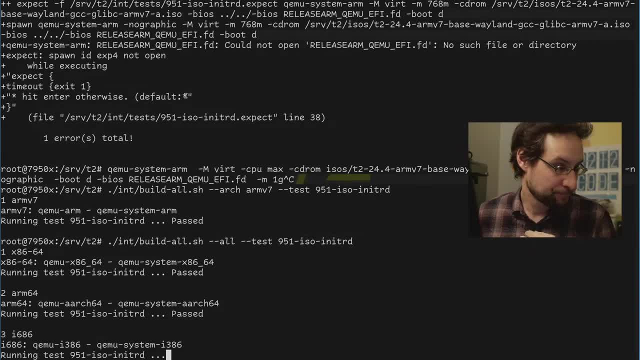 now that we have all Linux distribution working and tested to come.